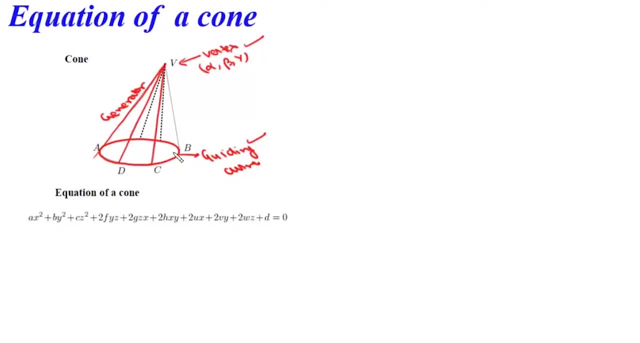 many generators, So all these lines, they are generators of this cone. Now equation of a cone. in 3D it is defined as ax square plus by square plus cz square plus 2fyz plus 2gzx plus 2hxy plus. 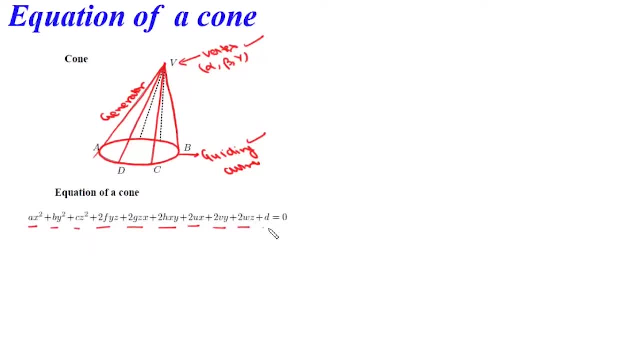 2ux plus 2vy plus 2wz plus d equals 0.. Now what we will do is we will try and prove equation of cone. it takes this one, So we already have this vertex. So we will write this alpha, beta and gamma and let us see equation of this guiding curve. 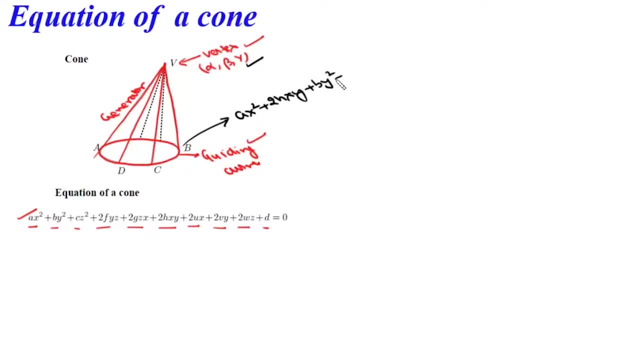 is ax square plus 2hxy plus, by square plus 2gzx plus 2fyz plus, gets equal to 0, and it lies in xy plane. z equals 0.. Now suppose direction ratios of generator. they are l, m and m. Now, once we try and improve those theás inter fra ground, we get the direction axis here and this is our definition of guidance curve. So this has the 10,. this provides a high frequency code and that means we are experts and this is correct, right, prank? I hope you like the idea of how exactly this information 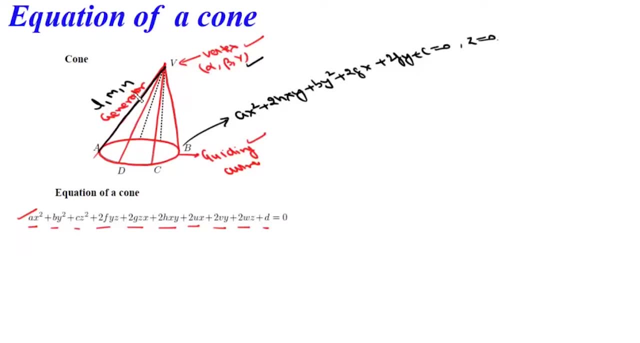 gets applied during competition and to find the empirical values. so let us get back to problem four. However, we have two equations of BA s- and that comes in the first one- which have this point and element. we can write equation of this line. So equation of this line will: 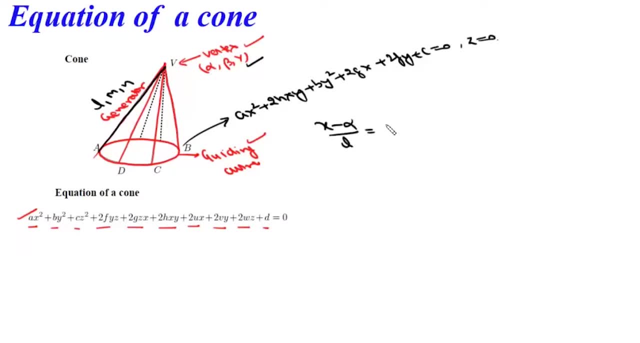 be: x minus alpha upon l equals y minus beta upon m, equals z minus gamma upon m. Now we need to find this point A, and on A, this z is 0.. Now if we put z as 0, we get x minus alpha upon l equals y minus beta upon m. that is equal to minus gamma upon m. So from here, 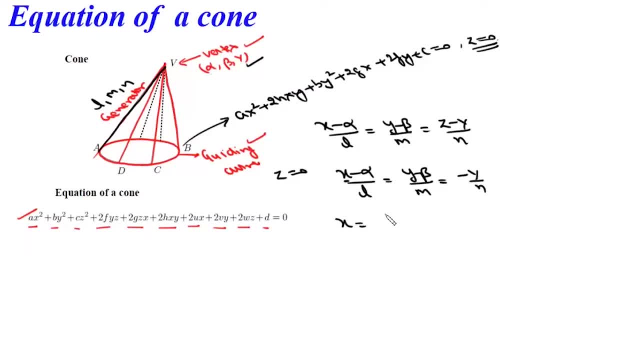 we can calculate this point x, and this point x will be: alpha minus gamma into l by m, and y equals beta minus gamma into m by m. So coordinate of this point A will be written as alpha minus gamma l by m, beta minus gamma m by m, comma 0.. Now this point A. it lies on: 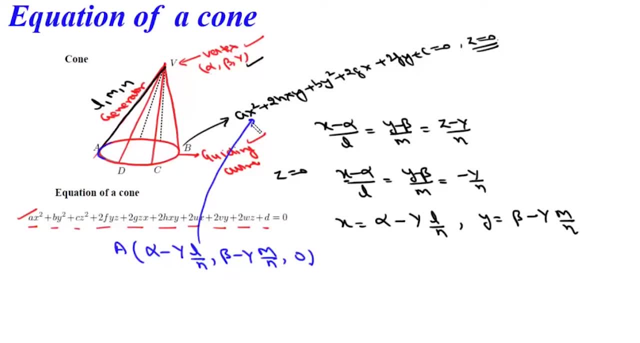 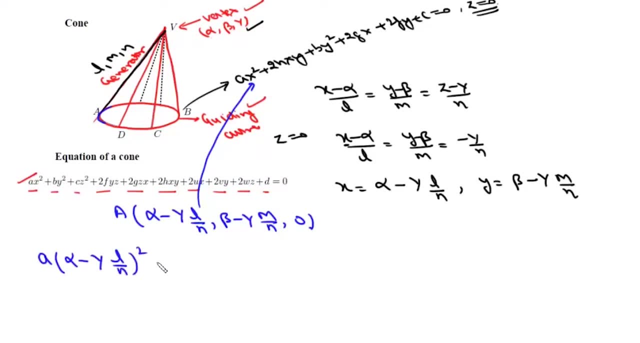 this guiding curve so it will satisfy its equation. so we will put it in this equation. Now we can write this as A into alpha minus gamma l by m, square plus 2h. alpha minus gamma l by m. beta minus gamma m by m. Now we can also write this: 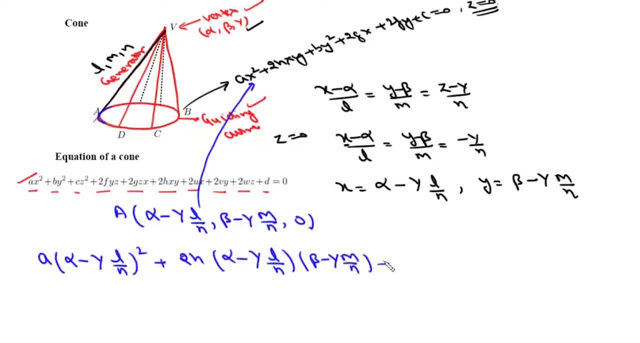 beta minus gamma m by m plus b. beta minus gamma m by m, whole square plus 2gh. alpha minus gamma l by m plus 2f. beta minus gamma m by m plus c equals 0.. of these two equations are playing from a Lorentzan model. 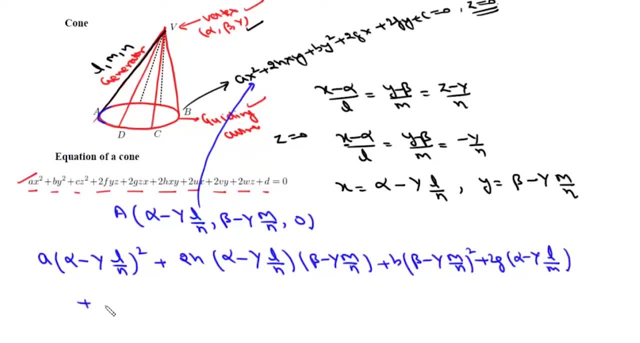 So we have obtained alpha minus gamma m by n into beta minus gamma m by m with here we will write: c equals 1.. so with this equation we can write: this is epsilon minus alpha minus gamma l by m plus 2f, beta minus gamma m by m. once again we will Press Start. 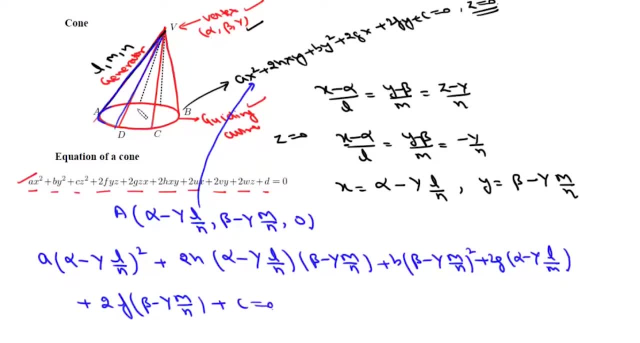 2. L, M and N. they will vary. Now, in order to find locus of these points X, Y, Z lying on these generators, what we need to do is we need to eliminate L, M and N. 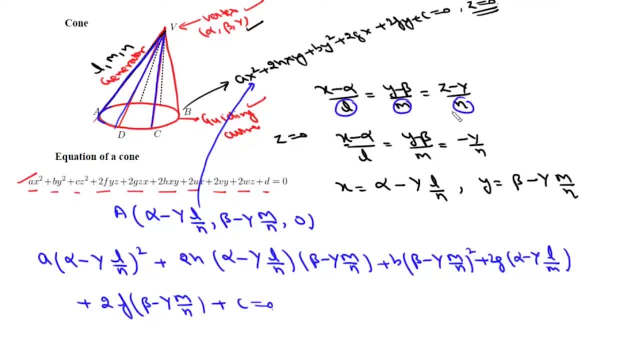 Now, from here, what we can do is we can write the value of L by N, and L by N is X minus alpha upon Z minus gamma. So we can write L by N as X minus alpha upon Z minus gamma, and we can also write M by N. 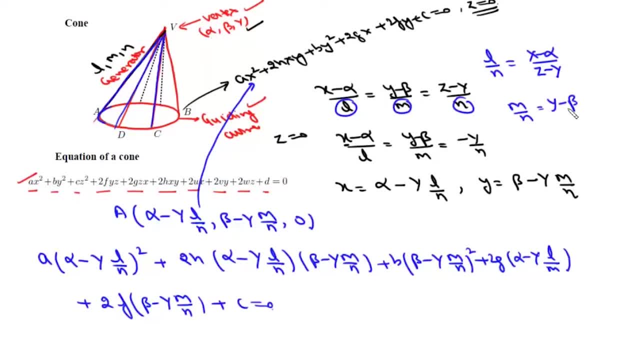 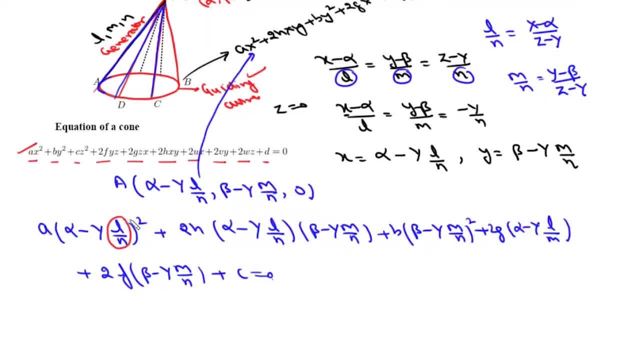 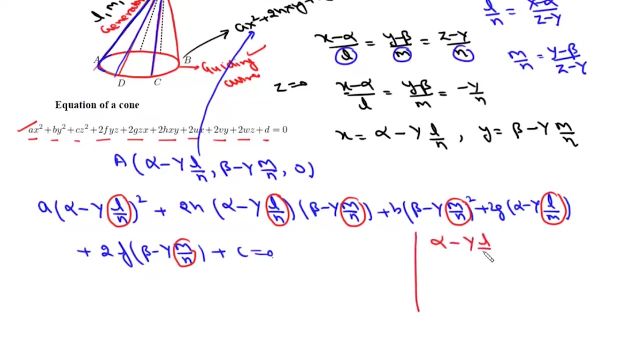 And M by N is Y minus beta upon Z minus gamma. So now we can put the value of L by N and M by N to eliminate L, M and N. Now if we write alpha minus gamma, L by N, so it will be alpha minus gamma. 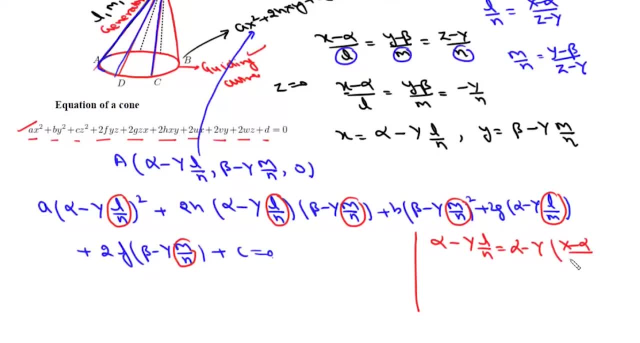 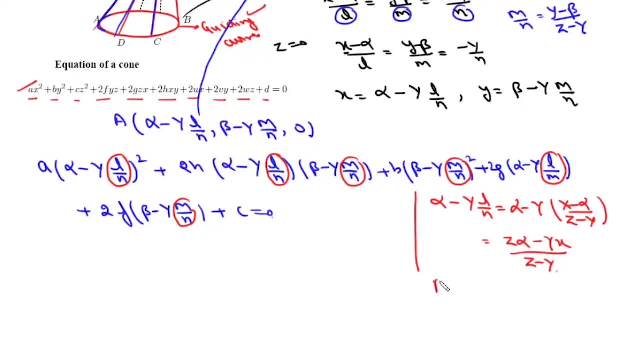 and this L by N will be X minus alpha upon Z minus gamma. Now it will be Z alpha minus gamma, X upon Z minus gamma. And in the same way we can write beta minus gamma, M by N is beta minus gamma. 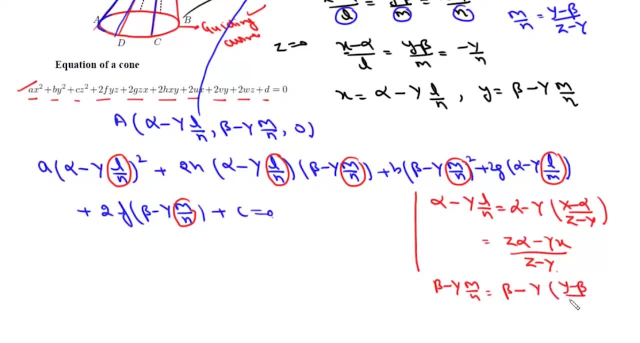 and M by N is Y minus beta upon Z minus gamma. So there will be beta Z minus gamma, Y upon Z minus gamma. Now, if we put it here, we can write this equation as now. if we simplify this equation, we'll get this equation in terms of X square, Y square, Z square. 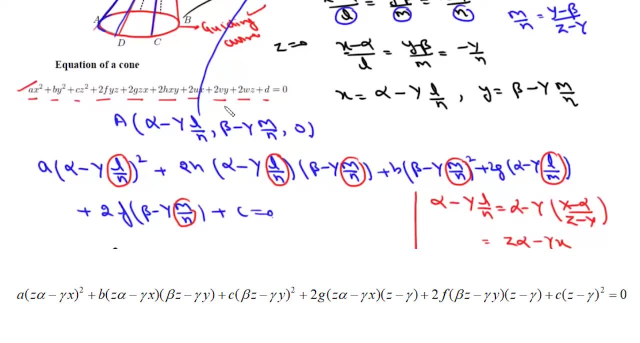 Then we'll also have YZ, XZ, XY and then XYZ plus constant tau. So basically standard equation of a cone. it'll look like AX square plus DY square plus CZ square plus 2FYZ plus 2GZX plus 2HXY plus 2UX plus 2VY. 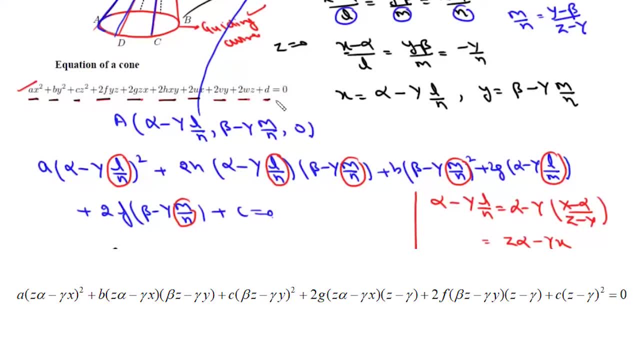 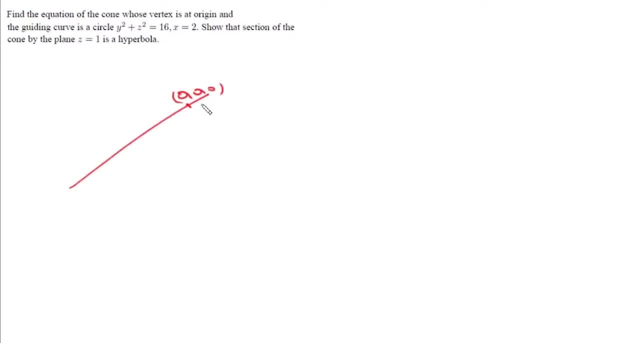 plus 2WZ plus D equals 0.. Now the question is: by the equation of cone, whose vertex is at origin and whose guiding curve is Y square plus Z square equals 16, and this is X equals 2FYZ. Now say direction ratios are L, M and N. 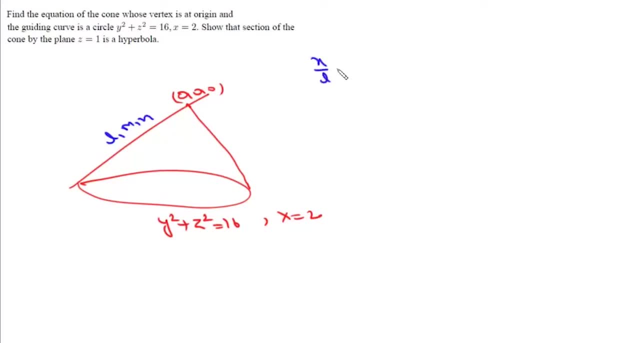 Then equation of this line will be: X by L equals Y by M, equals Z by N. Now this value of X is 2.. Now if we put X as 2, we'll get Y as 2, M by L and Z as 2, N by L. 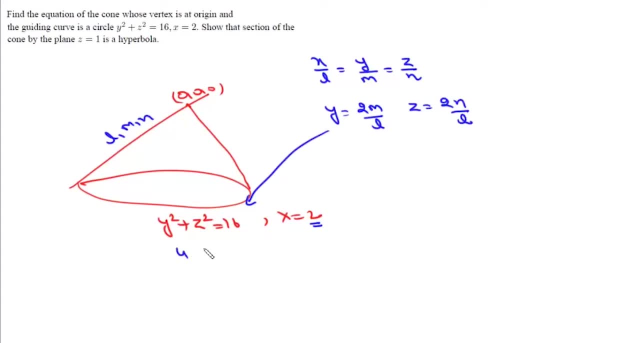 Now this point will love this curve, So it'll be 4.. M by L square plus 4, N by L whole square and it'll be equal to 16.. Now this 4 and 4 will cancel, so we'll get this 4 here. 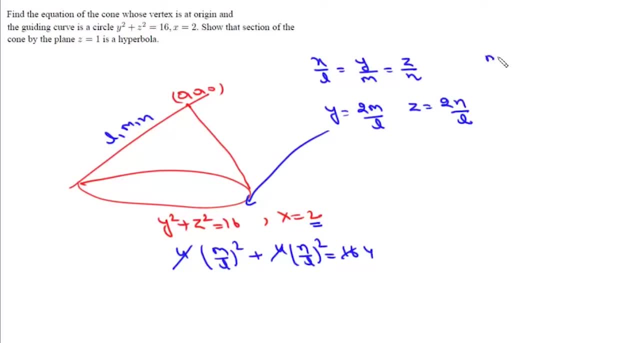 Now we need to eliminate L, M and N. Now, if we write M by L, M by L will be Y by X and N by L will be simply Z by X. Now we put these in this equation, So equation of this cone will be Y by X square. 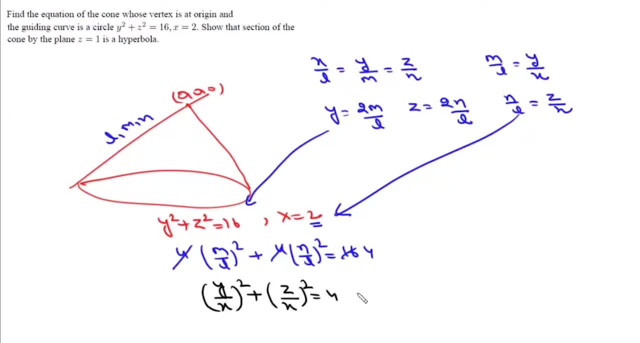 plus Z by X square equals 4, or Y square plus Z square equals 4X square. This is the equation of cone we are looking for Now. it says: show that section of the cone by this plane, Z equals 1, is a hyperbola. 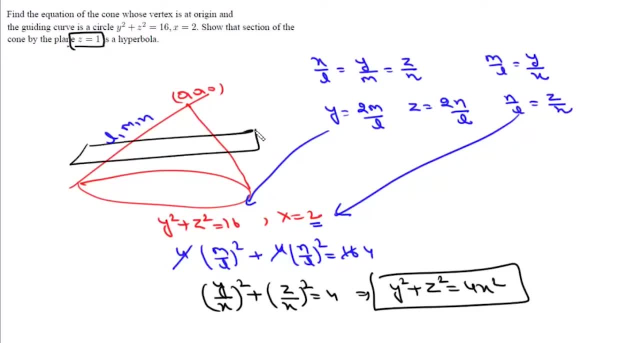 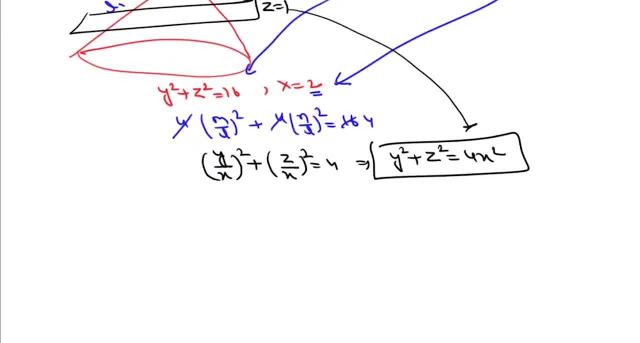 Now, if we take its intersection with this plane, Z equals 1, which means, if we put Z equals 1 in this equation, we can write this equation as 4X square, So we get minus Y square equals 1, which is nothing but equation of hyperbola. 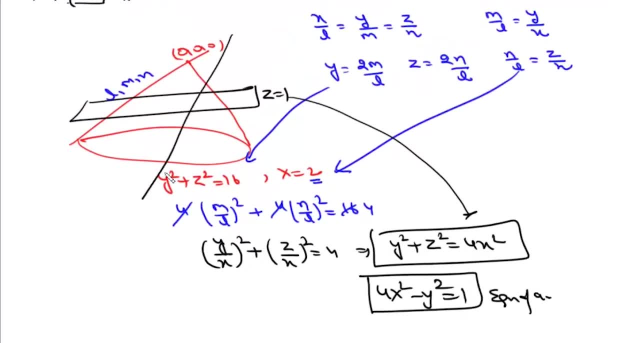 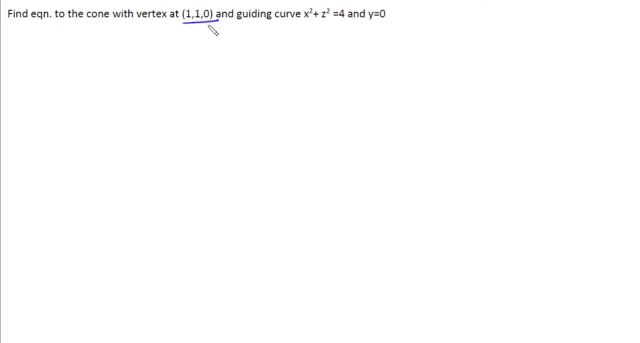 which means basically, this plane will intersect like this, so it will form a hyperbola. Now here the question is: find the equation to the cone with vertex at and guiding curve is X square plus Z square equals 4, and Y equals 0.. 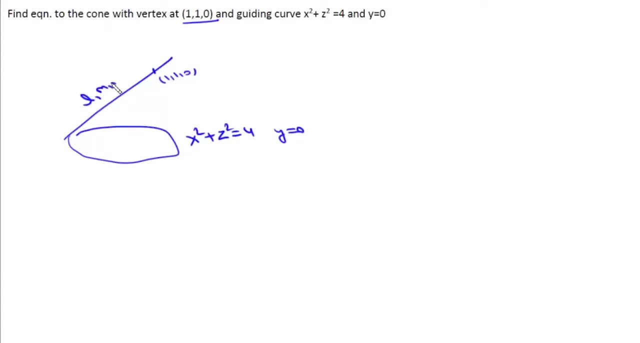 0.. assume direction. ratios of generator are l, m and n. then we can write this equation as: x minus 1 upon l equals y minus 1 upon m equals z minus 0 upon m. now it passes through this point: y equals 0. now if we put y as 0, we'll get x as 1 minus l by m and we'll get z as minus n by m. now we put 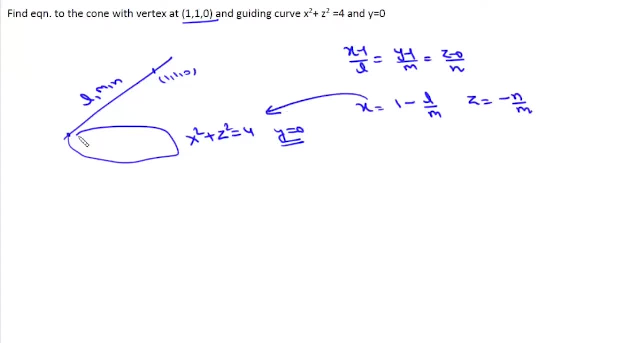 the value of x and z in this equation, because we are taking this point, which lies on this generator as well as on the guiding curve. we can write this equation as: 1 minus l by m square, plus minus n by m whole square, and it is equal to 4. now we need to eliminate l, m and n. now we know. 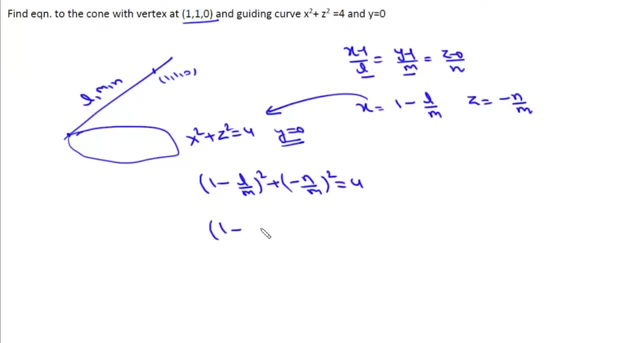 that l by m is x minus 1 upon y minus 1, so it will be 1 minus x minus 1 upon y minus 1 square, and n by m is z upon y minus 1 square, and it will be equal to 4. now this is y minus x, whole square. 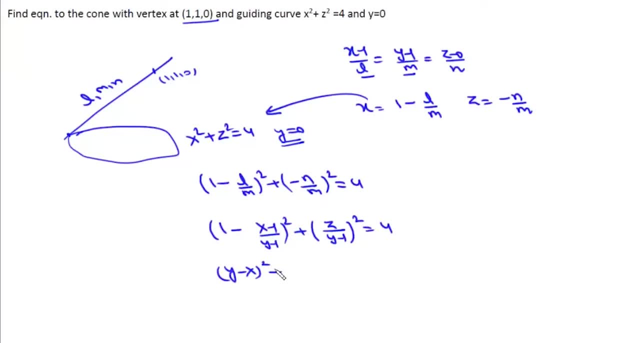 plus z square and it will be equal to 4 y minus 1 whole square. now we simplify this. we'll get this as: x square minus 3y square plus z square minus 2xy plus 8y minus 4 equals 0, and that is the equation of this required cone. now the question is find. 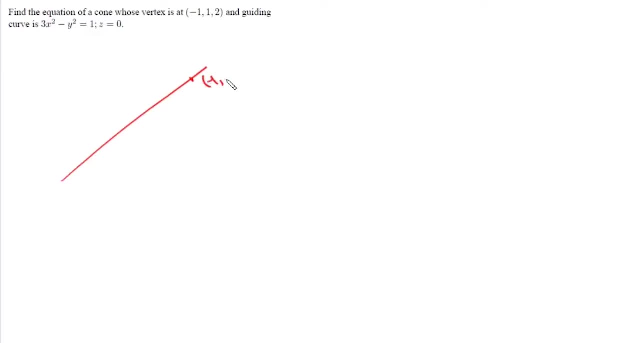 the equation of a cone whose vertex is at minus 1, 1, 2 and guiding curve is 3x square minus y square equals 1 and z equals 0. so we have this guiding curve. now let the direction ratios be l, m and n. 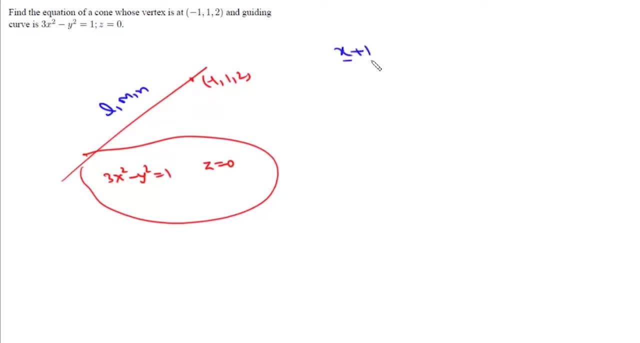 then equation of generator. we can write this as: x plus 1 upon L equals y minus 1 upon M equals z minus 2 upon M. Now for the guiding curve, z is 0. Now if we put z as 0, then we can get: 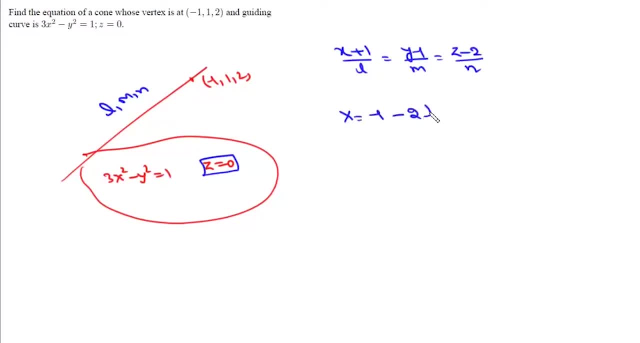 x equals minus 1 minus 2 L by M, and we get y equals 1 minus 2 M by M. Now these x and y's, they lie on this curve, so it will be 3, and this is 1 plus 2 L by M, square M minus and y is 1. 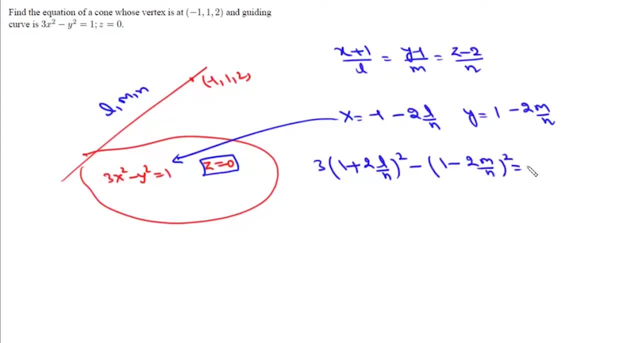 minus 2, M by M whole square and it is equal to 1.. Now we need to eliminate L, M and N. Now this L by N, it will be x plus 1 upon z minus 2, so it will be 3, and then 1 plus 2, x plus 1 upon. 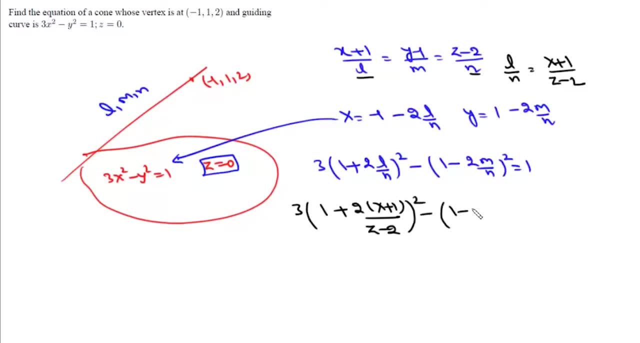 z minus 2.. z minus 2 square and minus this is 1 minus 2, and M by N is y minus 1 upon z minus 2 whole square and is equal to 1.. Now this is 3, and this is z minus 2, and 2x plus 2,, so it will be. 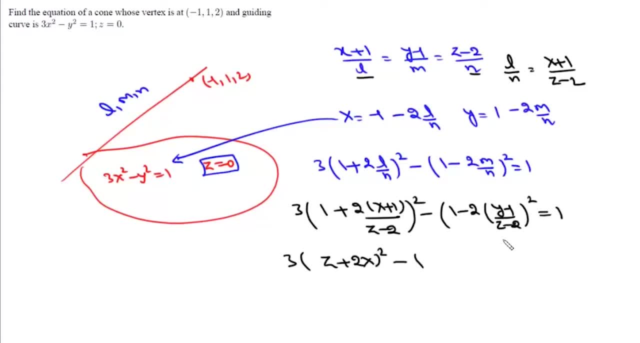 z plus 2x whole square and then minus. this is z minus 2, and minus 2y, so it will be z minus 2y whole square and it will be equal to z minus 2 whole square, and this is the equation of. 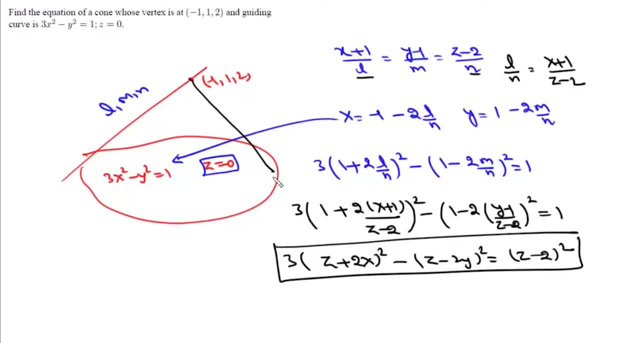 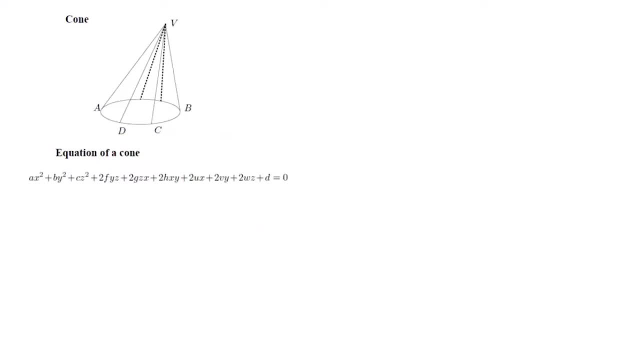 required cone for which this guiding curve and vertex is given. so now we know how equation of cone looks like. now what about equation of a cone whose vertex is at origin? so if we have a cone whose vertex it is at origin, and we'll prove that if vertex of this cone is at origin, then equation 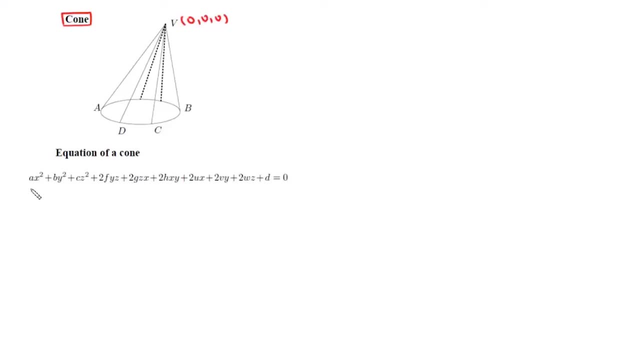 of a cone will be a homogeneous equation, so its equation will be ax square plus by, square plus cz, square plus 2f, yz plus 2g, zx plus 2h, xy and all of these they would be there in this equation. now say this point: it is given by x, y and z. and we have another point on this line which is: 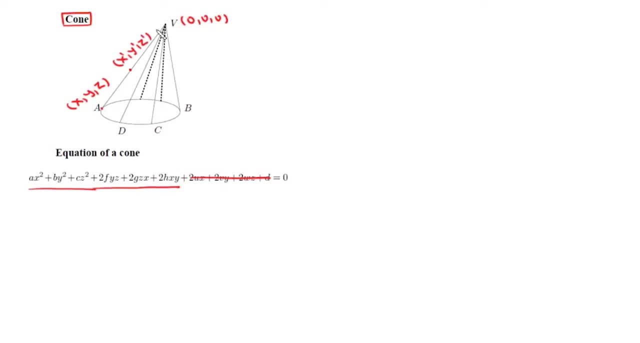 x dash, y dash and z dash. now we know that direction ratios. they are proportional. so x minus 0 upon x dash minus 0 will be equal to y minus 0 upon y dash minus 0 and z minus 0 upon z dash minus 0 and say it is equal to some lambda. 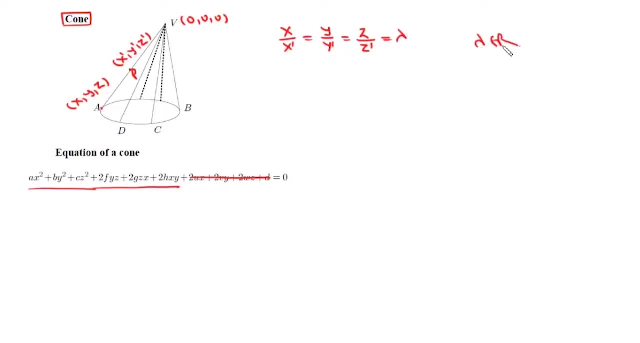 now here we have, lambda belongs to R, because as lambda varies, we'll have infinite points on the surface of this cone. now, this point a, we can write this as lambda x, dash, lambda y, dash and lambda z. this point a, it will lie on the cone. if we put the value of x, y and z, then we can write this equation. 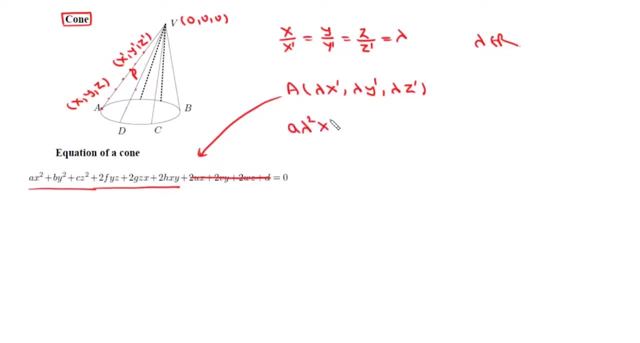 is a lambda square x dash square plus b lambda square y dash square plus c. lambda square z dash square plus 2f. lambda square y dash z dash plus 2g lambda square y dash z dash plus 2g lambda square z dash x dash plus 2h. lambda square x dash y dash plus 2u. lambda x dash plus 2v. lambda y dash plus 2w. lambda z dash and plus b equals 0. 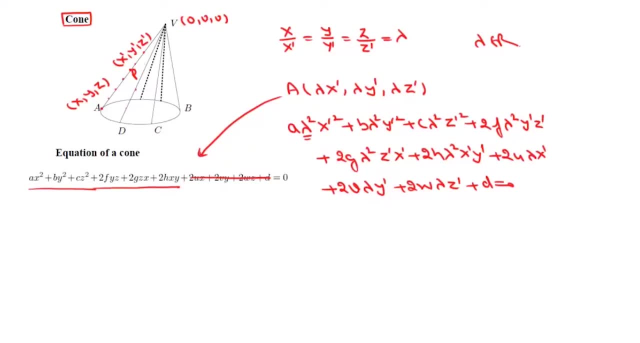 now it is a quadratic equation in lambda, so we can write this equation as: x dash square plus b y dash square plus c z dash square plus 2f y dash, z dash plus 2g z dash, x dash plus 2h x dash, y dash into lambda square, and then plus 2u x dash plus 2v y dash plus 2w z dash into lambda square. 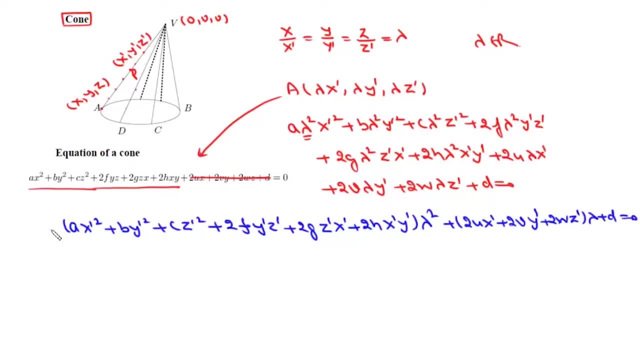 n plus d equals 0. now it is a quadratic equation in lambda, but then lambda belongs to r, so we just not have two values, we have infinite values of lambda, and if in a quadratic equation we have infinite solution, that means it becomes an identity. and it becomes an identity if a is 0, b is 0 and c is 0. 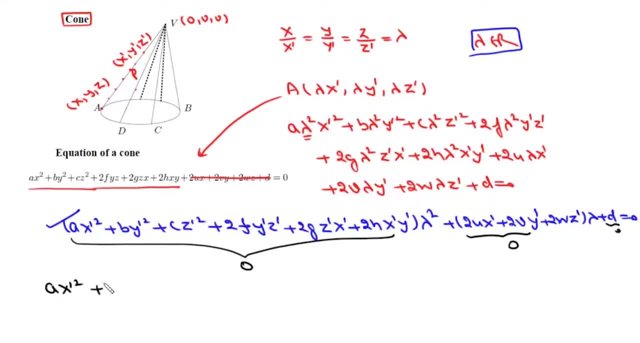 so from here we get this condition that ax dash square plus b y dash square plus c z dash square plus 2f y dash, z dash plus 2g z dash, x dash plus 2h, x dash, y dash. it must be equal to 0, and also 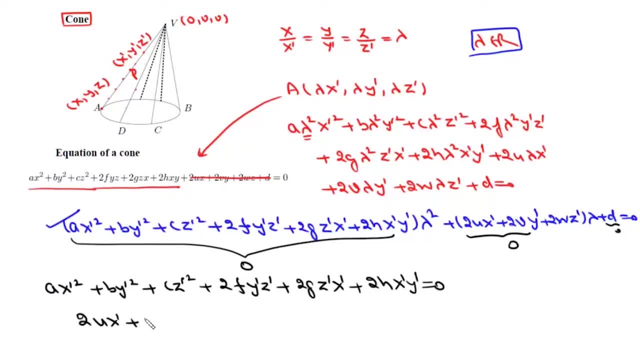 we will get this condition that 2u x dash plus 2v y dash plus 2w z dash. it must be 0 and d equals 0. so we have this condition: d equals 0. now from the second equation we will get equation of a plane, but then here we are looking for equation of a cone and not equation of plane. 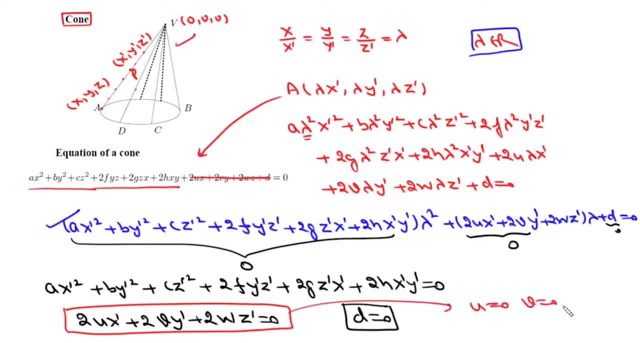 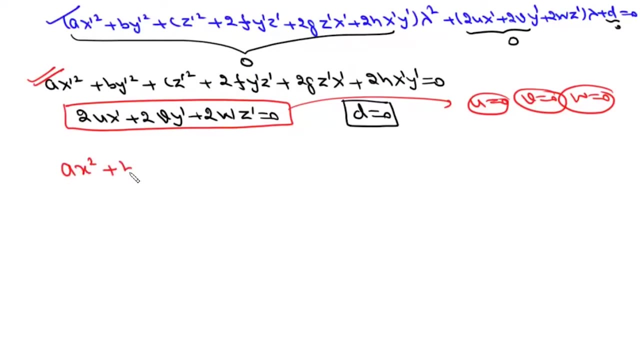 so here u must be 0, v must be 0 and w must be 0. so when we have u v and w and d 0, we are left with only this equation. so general equation of a cone will be given by ax square plus b y square plus. 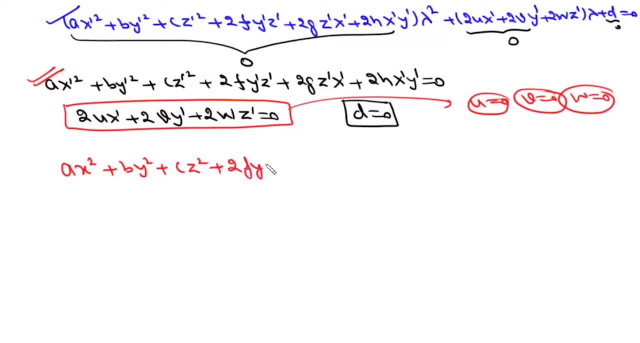 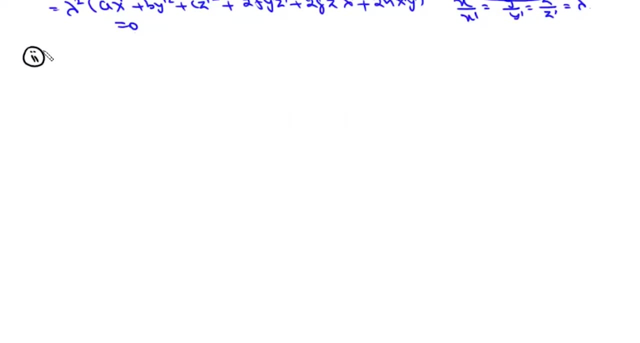 c z square plus 2f y z plus 2g z x plus 2h x y, and it will be equal to 0. now this second result that we will prove here is if we have equation of a cone passing through origin, and which is ax square plus b y square. 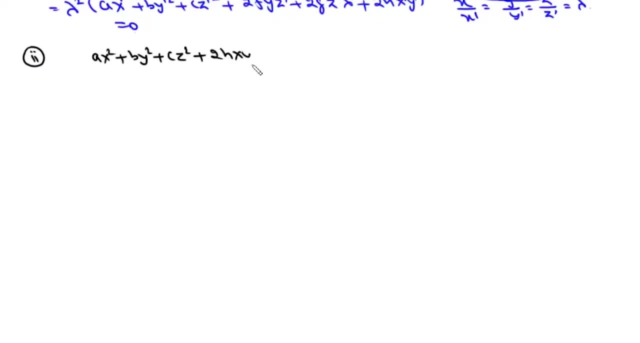 plus c, z, square, plus 2h, x, y, plus 2f, y, z, plus 2g x, y, zx equals 0 and we have a generator whose direction ratios are l, m and n. then basically direction ratios of this generator. they will satisfy this equation. 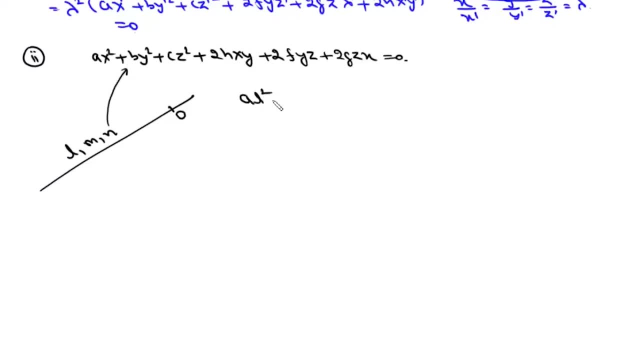 So we will prove that Al2 plus Bm2 plus Cn2 plus 2Hlm, plus 2Fmn plus 2Glm and it will be equal to 0, and this is a very important result which we will use in some questions. 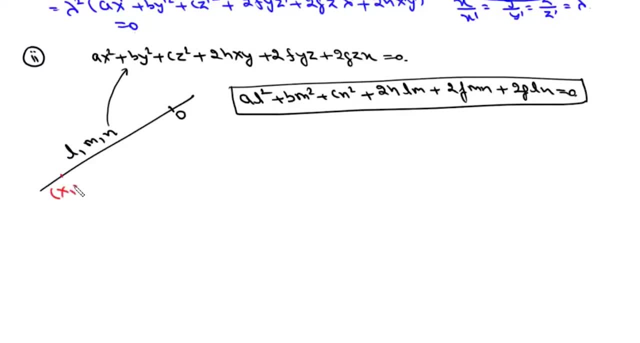 Now we take a point on this generator, say x, y and z, then we can write this equation as x upon l, y upon m and z upon n, and let it be equal to lambda. We can write coordinate of this point as lambda l, lambda m and lambda n. 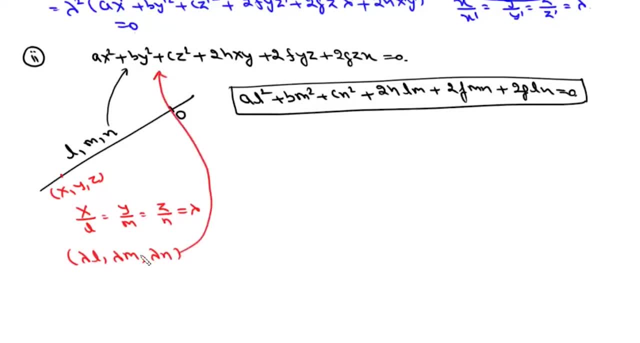 Now this point. it lies on this cone, so it will satisfy this equation. So we will write a and it will be lambda square l square plus b. lambda square m, square c. lambda square n square plus 2Hlm plus 2F. lambda square mn plus 2Glm, and it will be equal. 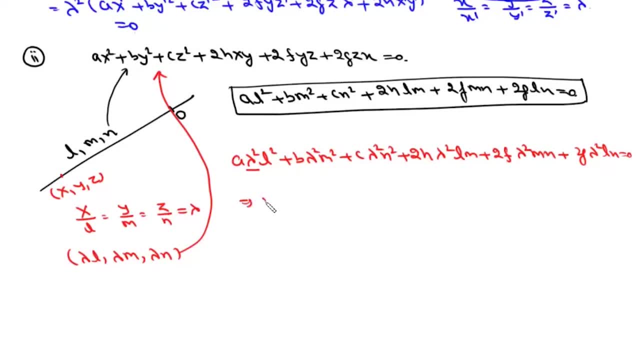 to 0.. Now we will take this lambda square common and then we will get Al2 plus Bm2 plus Cn2 plus 2Hlm, or lambda square Lm plus 2Fmn plus 2Glm. it must be equal. 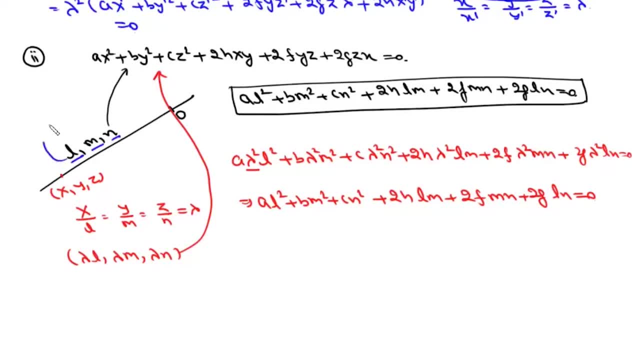 to 0.. If we write AL2 plus Bm2 with sum of del вз equal to 0, then all theコs are equal to 0. So direction ratios of any generator, they will satisfy equation of this cone. So if we have equation of cone as Sum fxyz equals 0 and direction ratios of any generator. 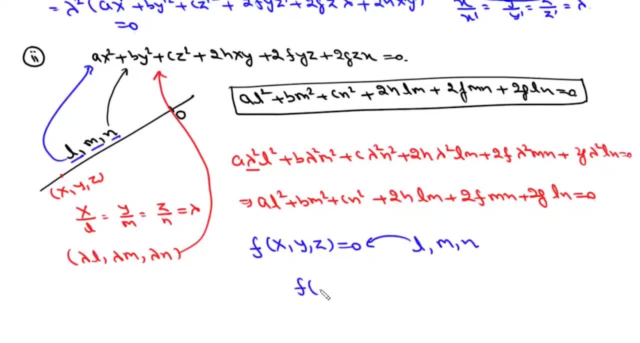 are Lmn And then we can simply say Lm 0ızlm. L, m and n will be equal to 0, and we can also use the result other way If L, m and n they are direction ratios of generator of a cone and they satisfy this. 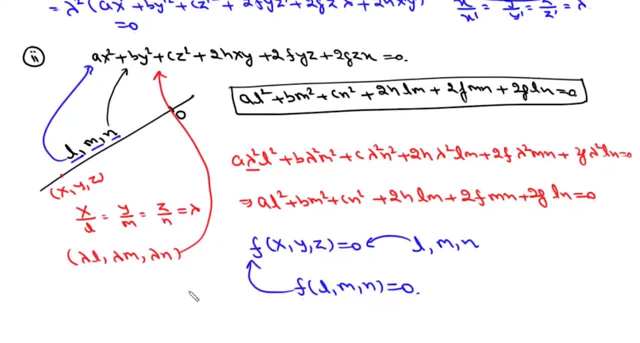 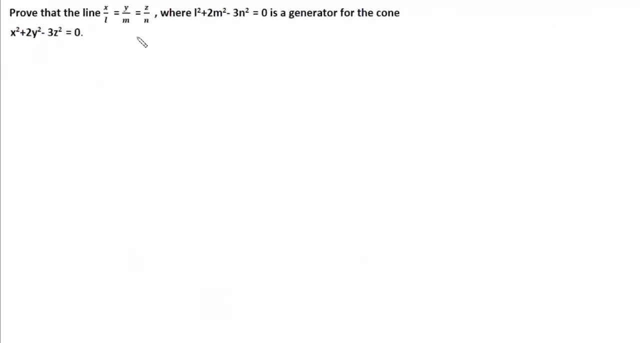 function. if L, m and n equals 0, then equation of cone is: F, x, y, z equals 0.. Now here the question is: prove that the line x upon L equals, y upon n, equals z upon n. where L square plus 2, m square minus 3, n square equals 0, is a generator for the cone x square. 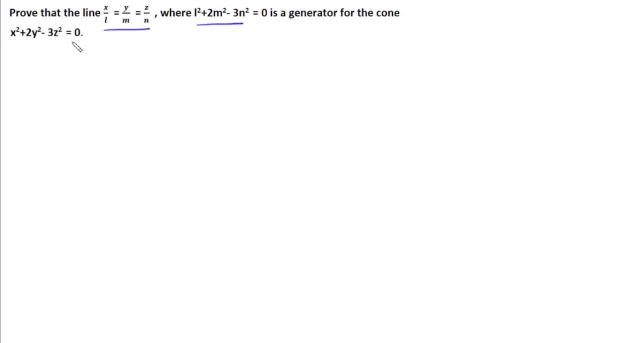 plus 2 y square, minus 3 z square equals 0.. Now this is equation of a cone passing through vertex 0, 0, 0 and origin lies on this generator. Now we know that if direction ratios of generator L, m and n, they satisfy some function phi. 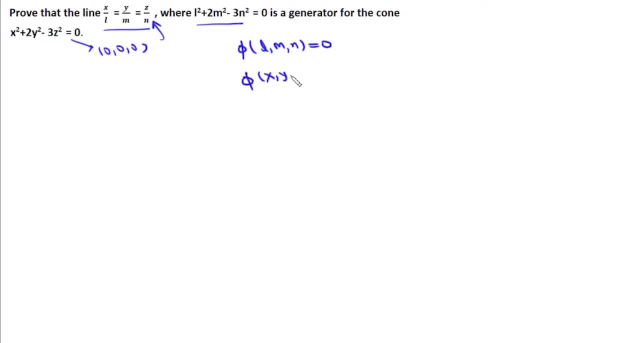 then equation of this cone is: phi, x, y, z equals 0.. Now, if we replace L with x, m with y and n with z, equation of this cone will be: x square plus 2, y square minus 3, z square equals 0, and which is what we need to prove in this. 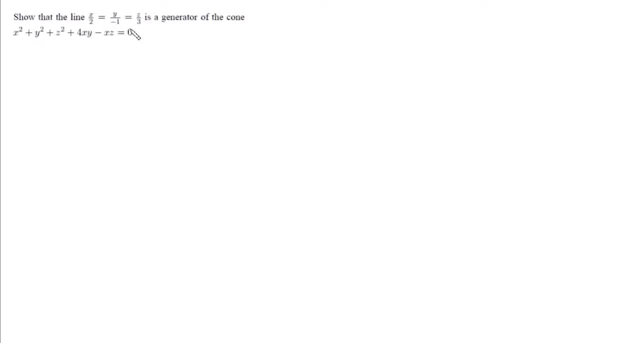 question. Now, here the question is: show that this line is generator of the cone. Now, since this curve is homogeneous and this line it also passes through origin, so point of this line, it satisfies this equation. Now we look at direction ratios of this line. direction ratios are 2, minus 1 and 3.. 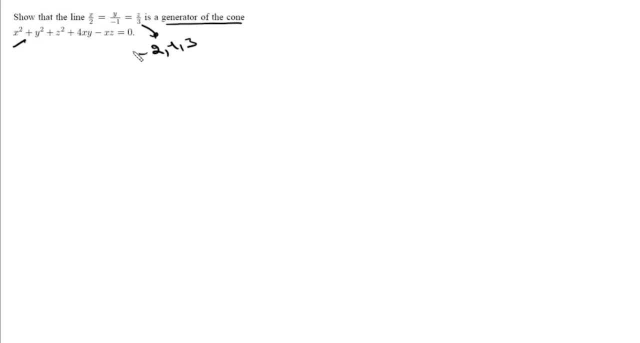 Now this line will be generator of this cone if direction ratios they satisfy this equation. So we need to check if L square plus m square plus n square plus 4, L m minus L n, it is equal to 0.. Now we will put this value. this is 4 plus 1 plus 9 and this is minus 8 minus 6.. 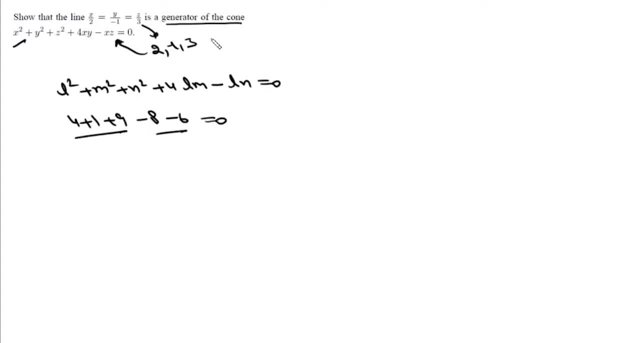 Now, this is 14 minus 14, and which is 0. That means this line. It indeed is 0.. Now we will prove our 3rd result, and which is equation of a cone whose vertex is at origin and which passes through 3 coordinate axis. 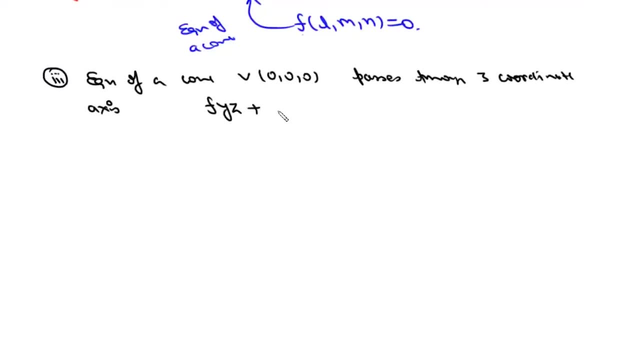 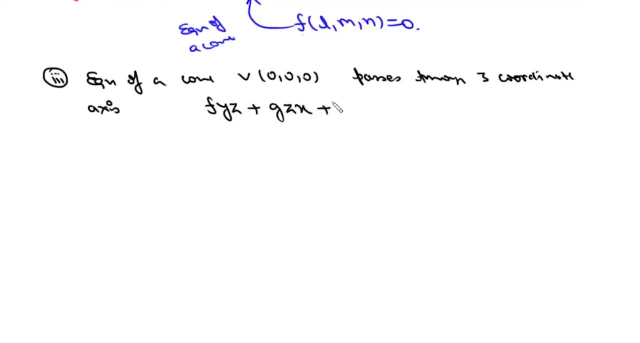 And we will put this value, which is 0.. And we will put this value, which is f? y, f y, z, greater than or equal to 0, especially if we eat the answer f? y, f y, z plus g, z, x, plus h x, y equals 0.. 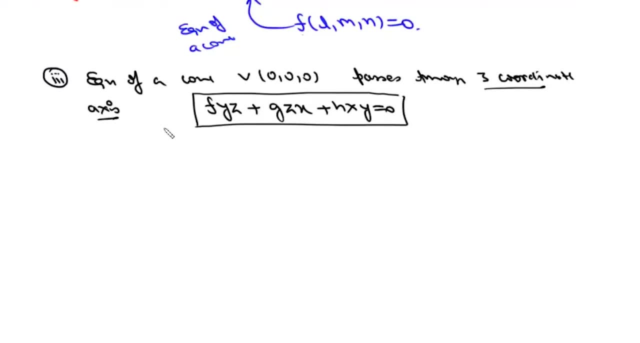 So this is equation of a cone with vertex at origin. and witch passes through all the three coordinate axis. So all the 3 coordinate axis will be generators of this cone. Now we already know that equation of a cone with vertex at origin. it is given by A x. 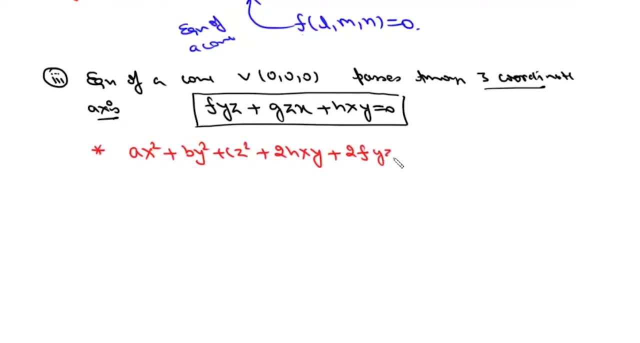 plus 2FYZ plus 2GZX equals 0.. Now one of the generators of this cone is x-axis And direction ratios of x-axis. they are 1,, 0,, 0. And we have proved that direction ratios of any generator. 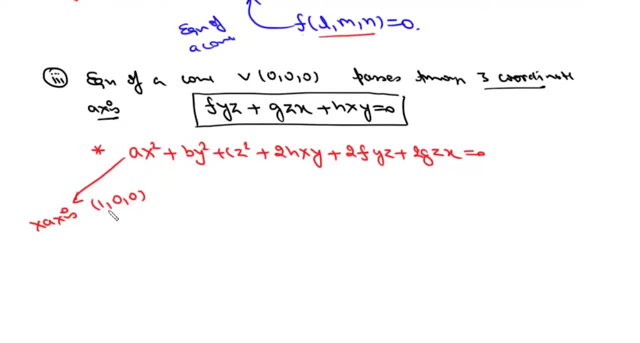 they'll satisfy this equation, So we'll put this value. So if we put L, M and N as 1, 0, 0, then we'll get A In A equals 0, for y-axis direction ratios are 0, 1, 0.. 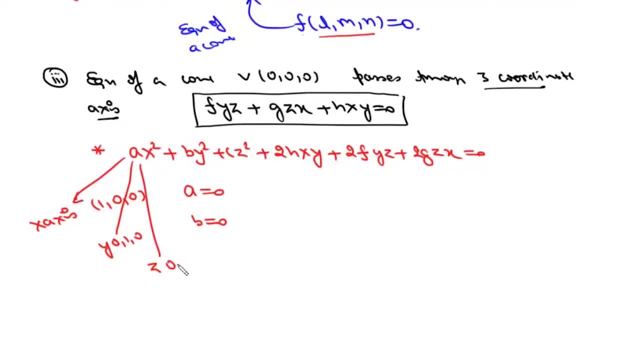 From there, we'll get B equals 0.. And for z-axis it'll be 0, 0, 1.. And we'll get C equals 0.. Now, if we put A, B and C as 0,, 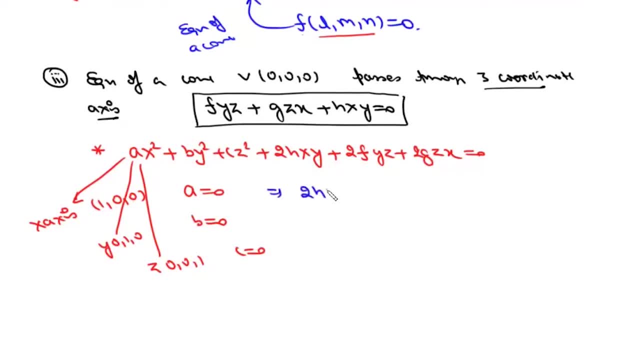 then we'll get equation of this cone as: 2HXY plus 2FYZ plus 2GZX equals 0.. We'll cancel this too, So this equation will be: HXY plus FYZ, YZ plus GZX equals 0.. 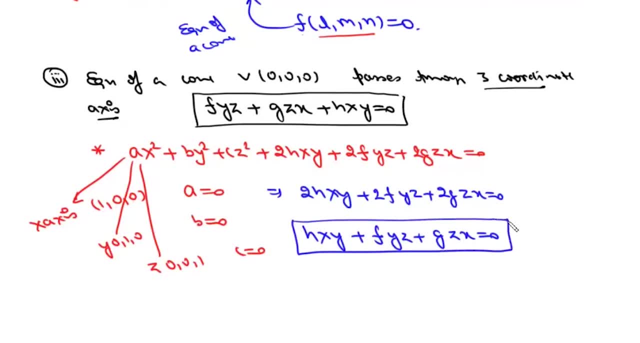 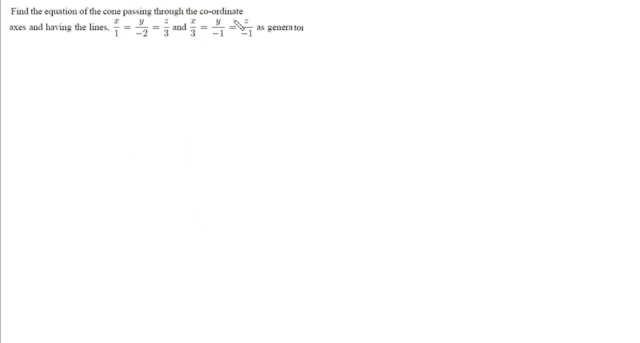 So this is equation of a cone with vertex at origin and passing through all the three coordinate Xs. Find the equation of a cone passing through coordinate Xs and having these lines as generators. Now we know that equation of cone passing through coordinate Xs. 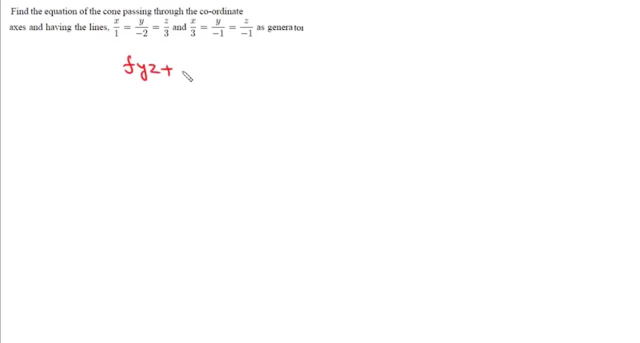 it is given by FYZ plus GZX plus HXY equals 0.. Now direction ratios of these first generator. they are 1, minus 2, and 3. And we know that direction ratios they satisfy this equation. 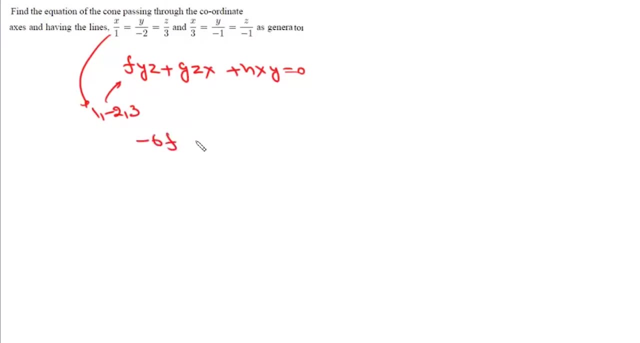 So we'll get this as minus 6F, plus 3G and minus 2H, and it'll be equal to 0.. Now direction ratios of this second line. they are 3, minus 1, and minus 1.. 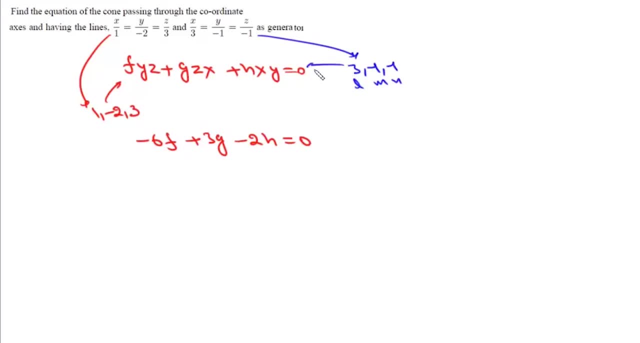 So they are L, M and N. Now they'll again satisfy this equation, So we'll get this as minus 6F plus 3G. Now ZX is M into N, So it'll be this F. 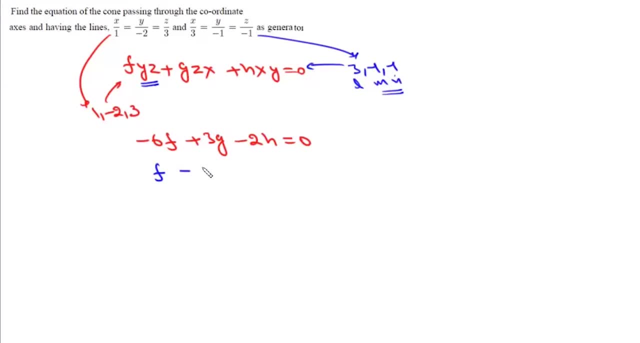 Now Z into X. Z into X is this minus 3.. So it'll be minus 3G. And then X into Y is minus 3H and it'll be equal to 0.. Now we can add this as F, G and H. 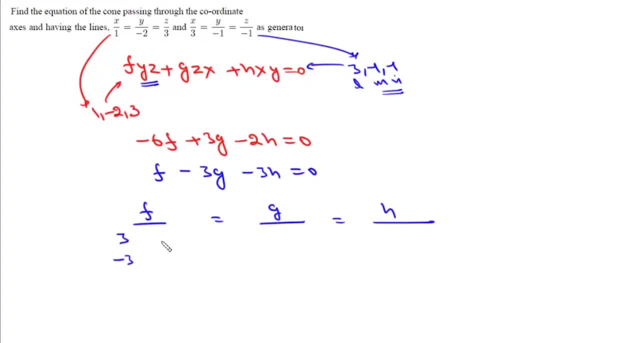 Now this is B1, B2.. So it'll be 3, minus 3, and C1, C2. So this is minus 2.. Minus 3.. Now this is minus 2, minus 3.. 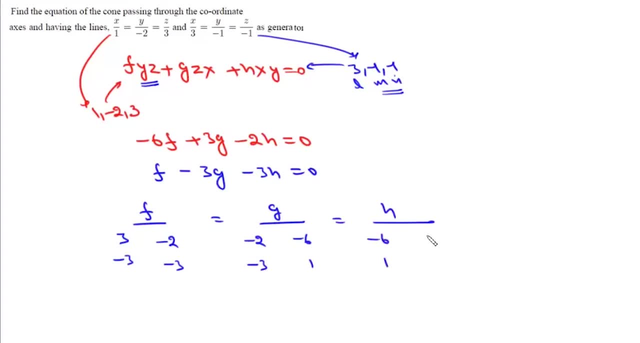 This is minus 6, 1, minus 6, 1, and 3, and minus 3.. So it'll be minus 9, minus 6.. So F upon minus 15.. G is minus 2, minus 18, minus 20.. 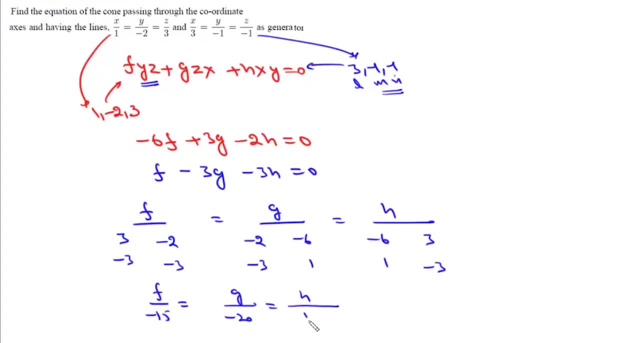 And H is 18, minus 3, 15.. So these F, G and H, they're proportional to minus 15, minus 20, and 15.. Now we take them as some lambda. Then we can write this F as minus 15 lambda. 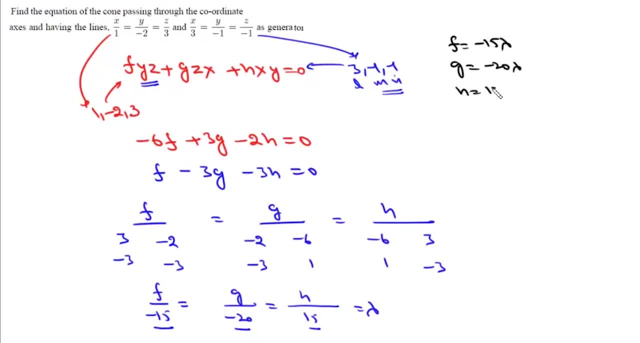 G as minus 20 lambda And H as some 15 lambda And if we put them in this equation we can actually take minus 5 lambda common. So if we take minus 5 lambda common, so there'll be 3YZ plus 4ZX minus 3H. 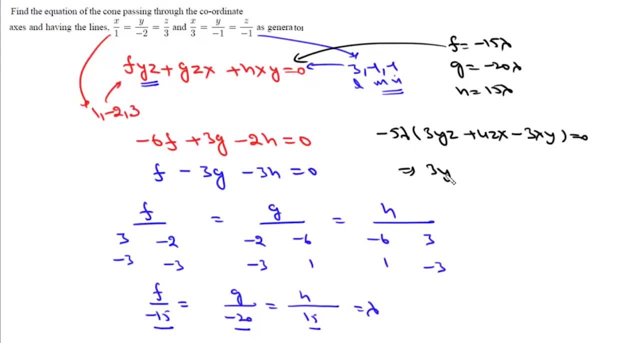 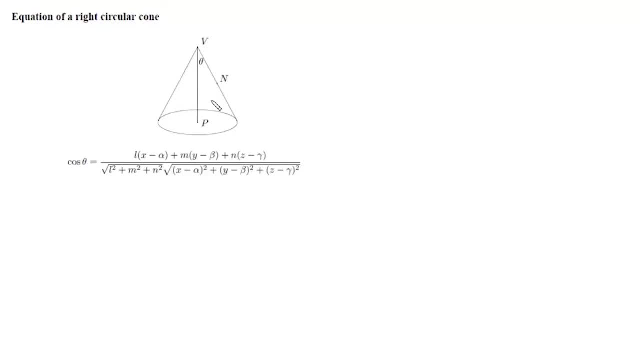 Minus 3XY equals 0. So equation of this cone will be: 3YZ plus 4ZX minus 3XY equals 0.. Now we'll come to a right circular cone. Now, basically, a right circular cone is a surface generated by a straight line. 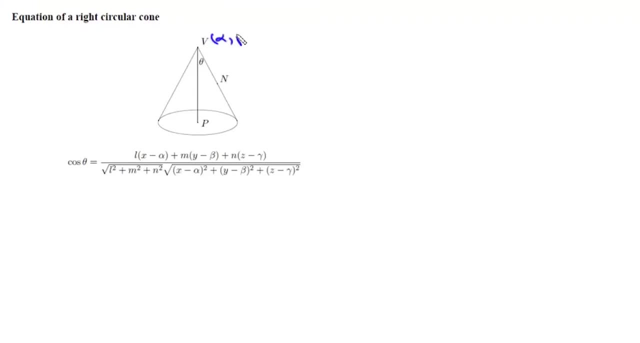 passing through a fixed point, which is vertex, say alpha, beta and gamma, making a constant angle, theta, with a fixed straight line passing through a given point. So this fixed straight line, and we call this line as axis of a cone. 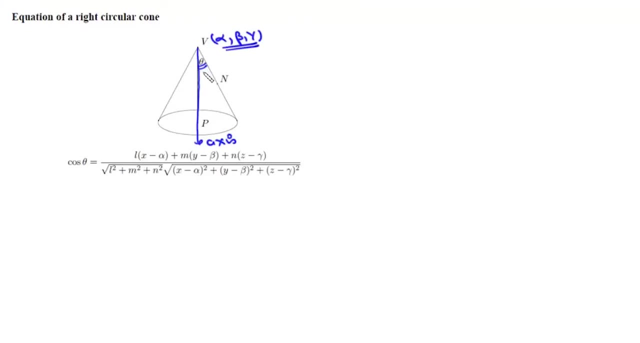 So we'll be given vertex, alpha, beta, gamma, We'll be given this half angle theta And then we'll be given this fixed straight line which is your axis of cone. Now we need to write equation of a right circular cone. 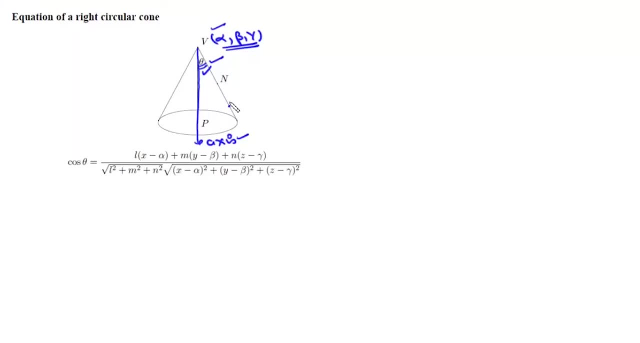 Now for this. what we'll do is we'll take up a general point on the surface and we'll take this point as XY and Z and say this point is 80. Now we can write direction. ratios of VA. 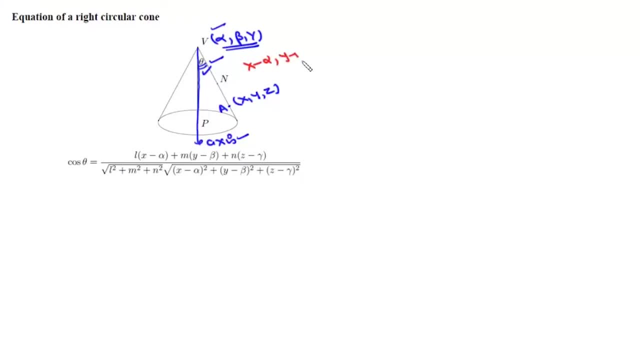 Direction ratios of VA are X minus alpha, Y minus beta, M, Z minus gamma. And we'll also be given equation of the axis or direction ratios of the axis. And suppose direction ratios of the axis are L, M and N. 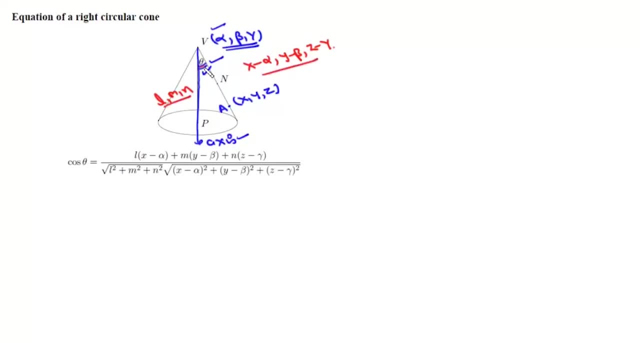 Now, once we have direction ratios of two lines, we can find angle between them And it'll be given by cos theta and it'll be equal to A1, A2.. So it'll be L X minus alpha, plus M Y minus beta and plus N Z minus gamma upon under root of. 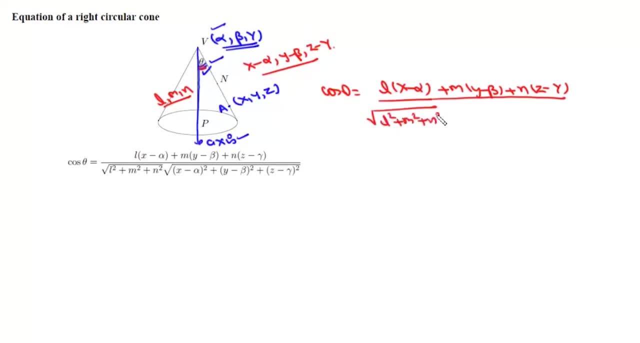 L square plus M square plus N square, into under root of X minus alpha square, Y minus beta square and Z minus gamma square, And this is the equation of a right circular. So if we square it, we can add this as cos square theta into L square plus M square. 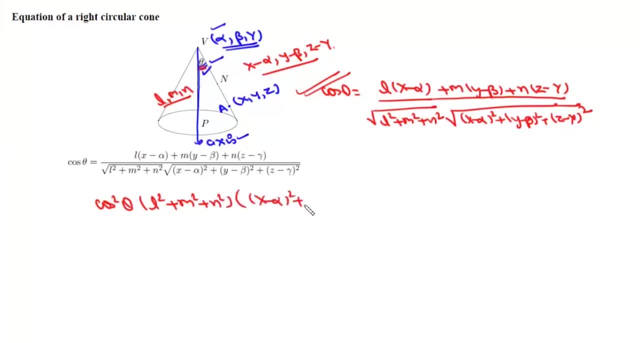 plus N square into X minus alpha square, Y minus beta square and Z minus gamma square, And here it'll be LX minus alpha plus M, Y minus beta plus N, Z minus gamma whole square, And this is the equation we are looking for. 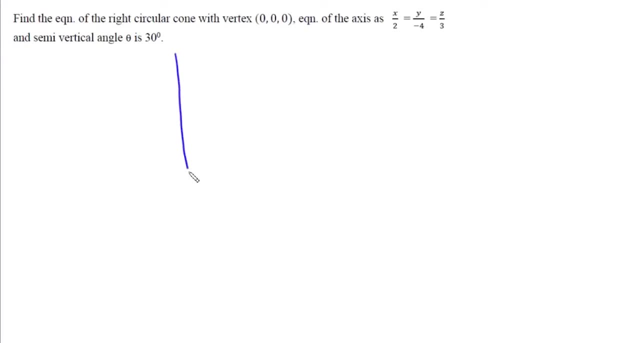 Now here the question is: find the equation of a right circular cone with vertex at origin and X is in the direction of 2, minus 4, and 3, and this semi-vertical angle as 30 degrees. Now let us do any point, say P XYZ on the surface of this cone. 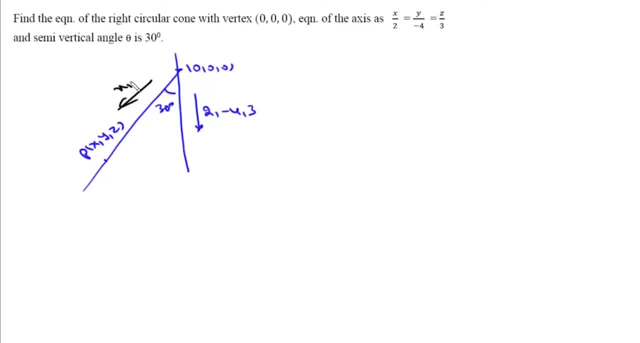 Now direction ratios of this line we can find. Now let us do any point, say P, XYZ, on the surface of this cone. ratios of this line, they are x, y and z, and here direction ratios are 2 minus 4 and 3. 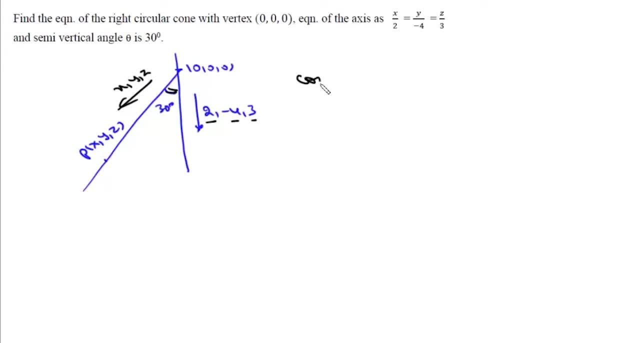 and angle between them is 30 degrees. so we can write cos 30 as 2x minus 4y plus 3z. upon now, this is under root of x square plus y square plus z square, and then into now, this is 16 plus 9, 25, 25 plus 2 is 25 plus 4 is root 29 and is equal to cos 30. 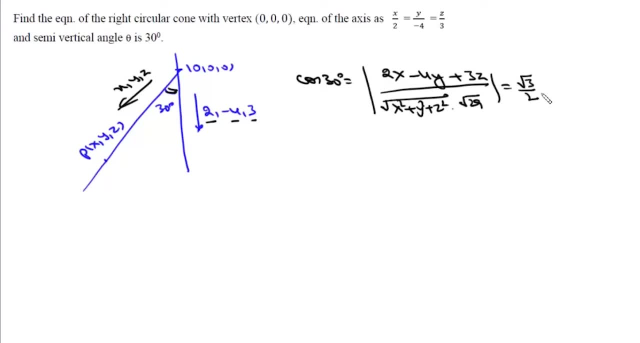 and cos 30 is under root 3 by 2. now we square it. we can write this as 4 into 2x minus 4y plus 3z whole square, and it will be equal to 29 into 3 into x square plus y square plus z square. so it will be this: 4 into 2x minus 4y. 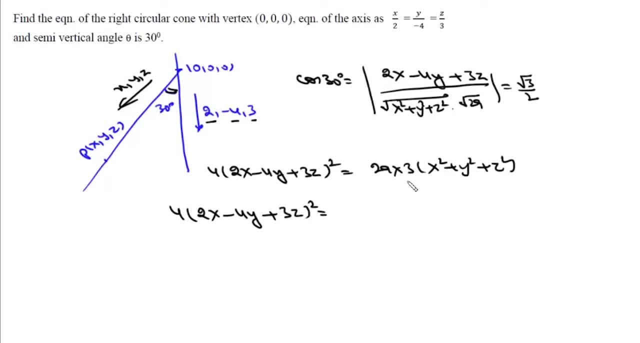 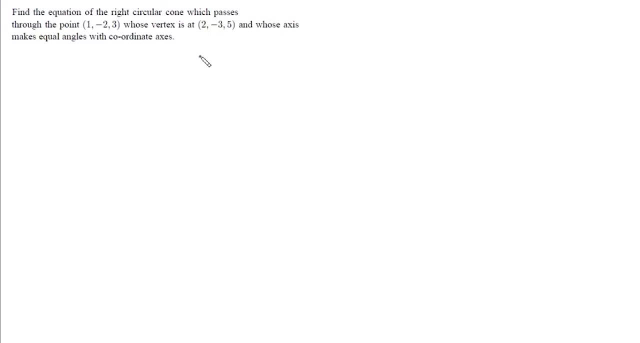 plus 3z whole square and 29 into 3 is 87 x square plus y square plus z square, and that is the equation of this right circular cone. right equations find the equation of a right circular cone whose vertex is at 2, minus 3 and 5 and which passes through this point which is 1, minus 2 and 3, and whose 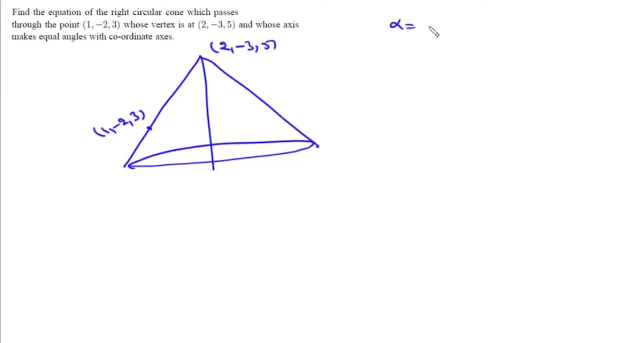 axis makes equal angle with coordinate axis. So if it makes equal angles with coordinate axis, then alpha equals beta equals gamma. that means direction cosines. they will be same. l equals m equals n. Now l square plus m, square plus n, square is 1. that means value of l, m and n is either. 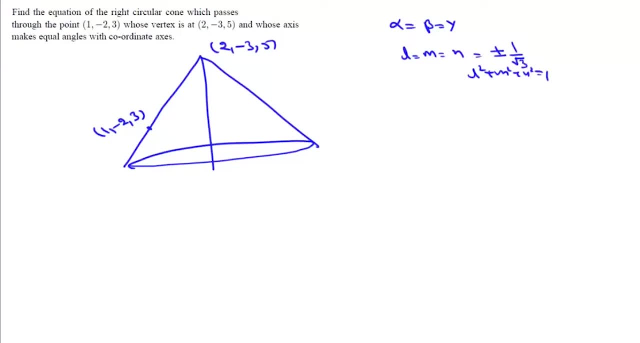 plus 1 by root 3 or minus 1 by root 3.. So from here we will get direction ratios of this axis, and they are 1, 1 and 1.. Now, first we will find this half angle using dot product. 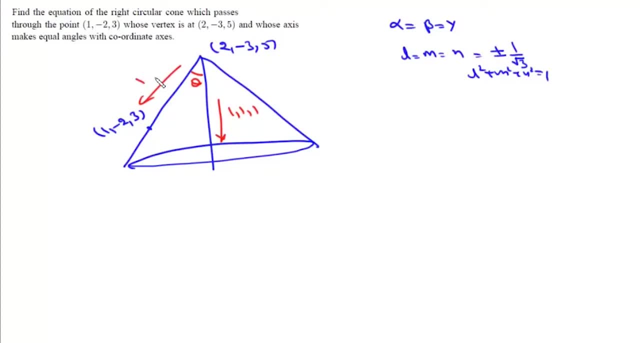 Now direction. ratios of this line will be 1, minus 1 and 2. then cos theta will be minus 1.. So 1, minus 1 plus 2 upon under root 6, and this is root 3, so it will be simply under. 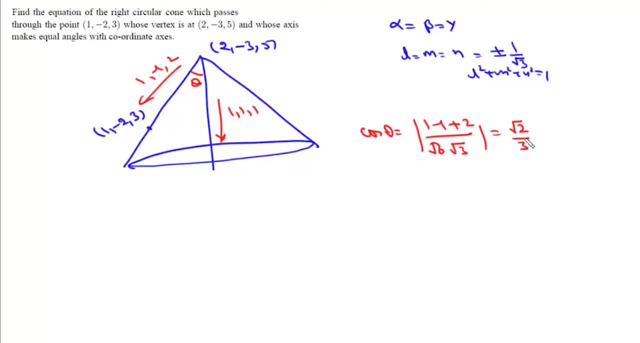 root 2 by 3.. So this half angle is cos inverse root 2 by 3.. Now we take any general point, say x, y and z, then we can write cos theta which is under root 2 by 3 as dot product between this vector, which is 1, minus 1 plus 2 by root 3.. 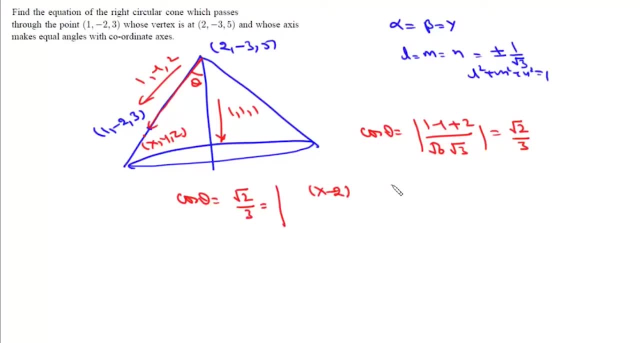 So this half angle is cos inverse root 2 by 3.. Now we take any general point, say x, y and z, then we can write cos theta which is under root 2 of x. If we look at the den Metro in my simulation it will be x minus 2, y plus 3 and z minus. 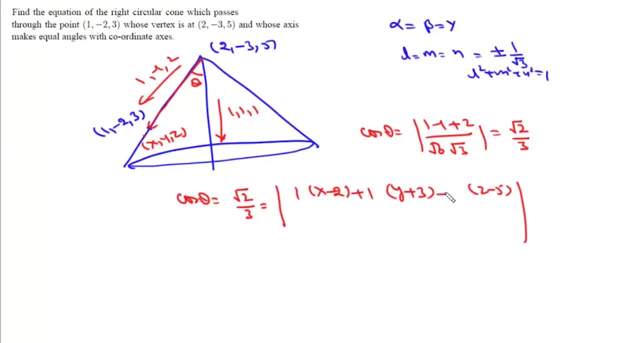 5, and then this is 1, 1 and 1, so it will be plus 1 plus 1 and plus 1. divided by now, this is root 3 and this is x minus 2 square plus plus z minus 3 square plus z minus. 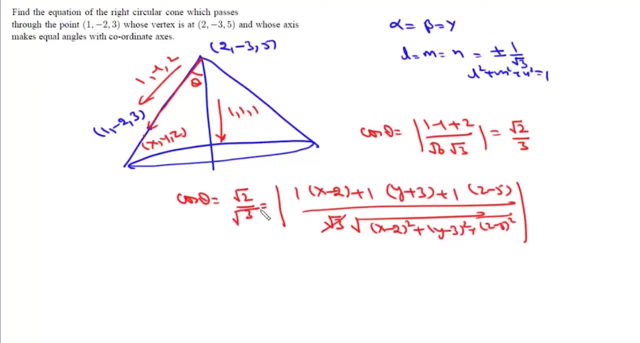 5 square. Now this root 3 and root 3 will cancel and we square it. we can write 2 into x minus 2 square plus z minus 5 square square plus y plus 3 square, because we have plus here: y plus 3 square plus z minus 5 square. 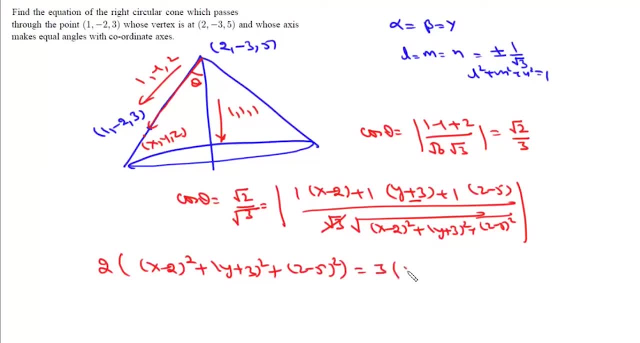 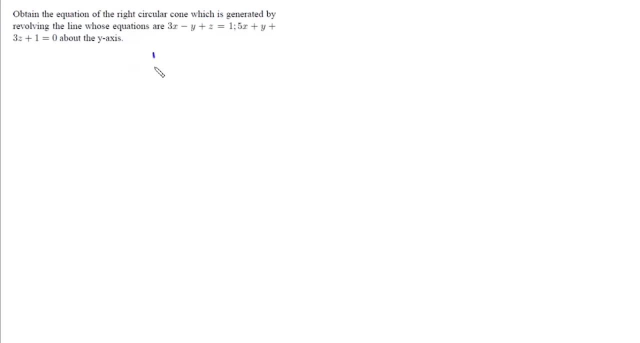 and it will be equal to 3 into, and this is x plus y plus z and here will be minus 4 whole square, and this is the equation of this right circular cone. Next equation is: obtain the equation of right circular cone which is generated by revolving. 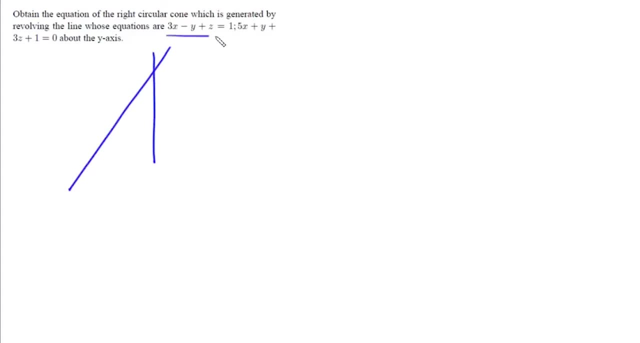 the line whose equations are: 3x minus y plus z equals 0 and 5x plus y plus 3z plus 1 equals 0. about y axis. So you are talking about this y axis. now, on y axis, x and z, they are 0. now we put x and 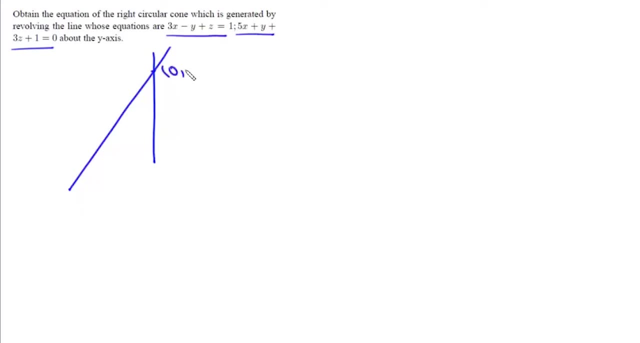 z at 0, we will get y as minus 1, so this vertex of this cone will be 0 minus 1 and 0, and axis of this cone will be along y axis. so direction ratios are 0.. Now we need direction ratios of this generator as since this line, it is line of intersection. 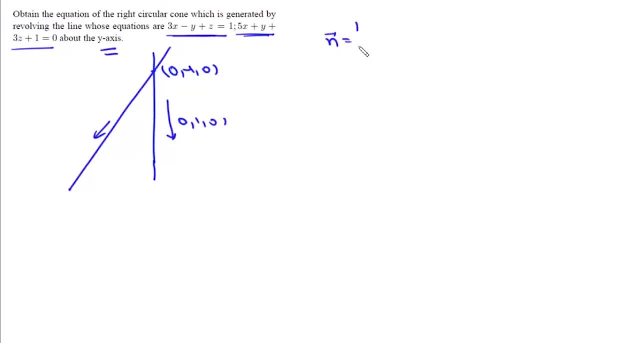 of two planes. we can find its direction ratios using cross product. so this is I, j and k, and here it is 3 minus 1 and 1. so this is 5 and 1 and 3. now this is minus 3 minus 1. 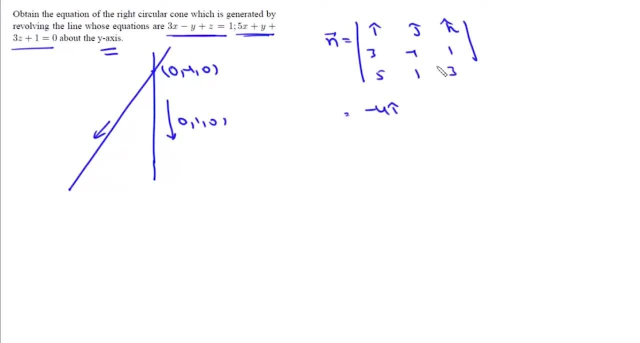 there will be minus 4i. now this is 9 minus 5 minus 4j. and here will be 3 plus 3 plus 1.. 5, 8 plus 8k. So direction ratios of this line. they are 1, 1 and minus 2.. Now once. 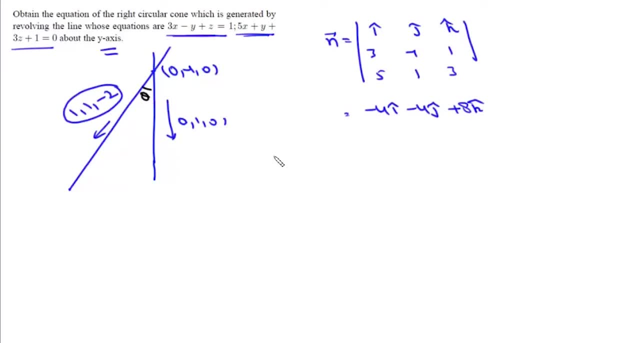 we have direction ratios, we can find this half angle theta. Now cos theta will be 1 upon under root of now. this is root 6 and this is 1.. Half angle is cos inverse 1 by root 6.. Now we take any general angle which is x, y and z. we can write cos theta which 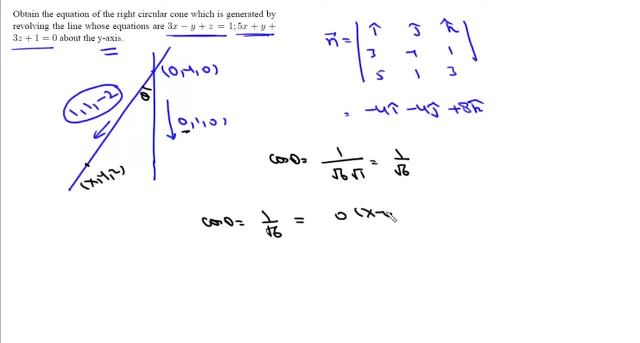 is 1 by root 6, it will be 0 into x minus 0 plus 1 into y plus 1 plus 0 into z minus 0. upon now, this is 1, and this is under root of x square plus y plus 1 whole square, and 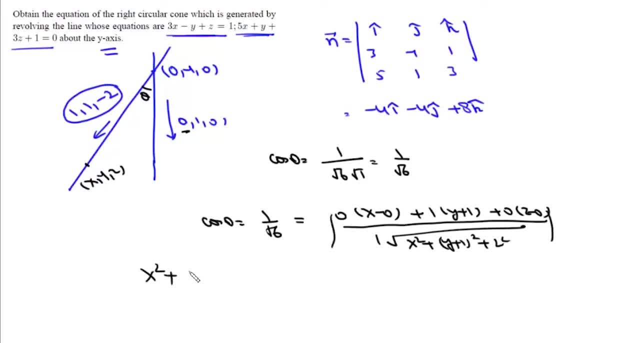 plus z square. Now we square it. we can write x square plus y plus 1 whole square plus z square, it will be equal to 6.. y plus 1 whole square, and that is the answer to this question. Now there will be some questions. 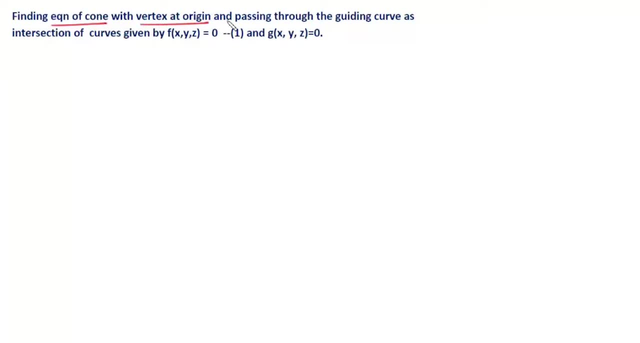 where we need to find equation of a cone with vertex at origin and passing through the guiding curve as intersection of the curves given by f x y z equals 0 and g x y z equals 0.. Now what we will do is, using these two equations, we will make the curve homogenous. 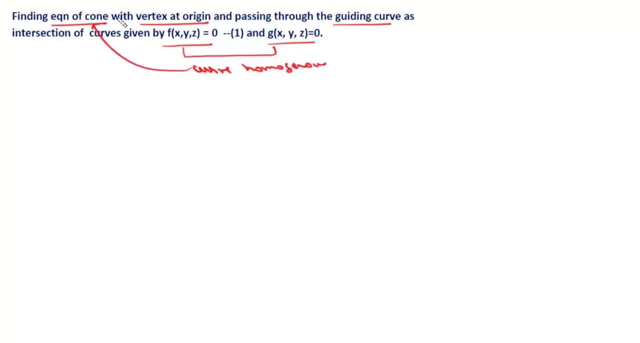 and this homogenous equation in second degree will represent equation of this cone. Now say, for example: find the equation of a cone with vertex at origin whose guiding curve is given by x square plus y square plus z square minus 2x plus 2y plus 4z minus 3. 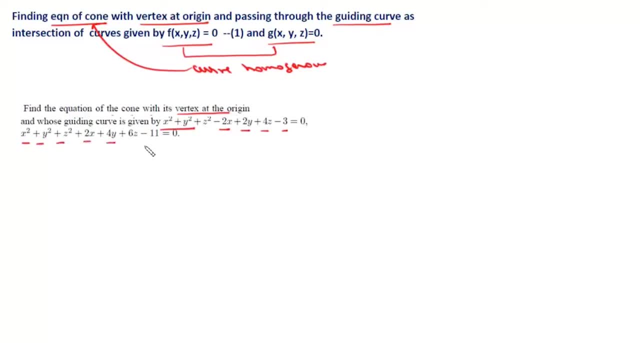 and x square plus y square plus z square plus 2x plus 4y plus 6z minus 11 equals 0.. Now, in order to make the curve homogenous, we have two options now. one is we can directly subtract this first equation from the second equation. then we can write 4x plus 2y plus. 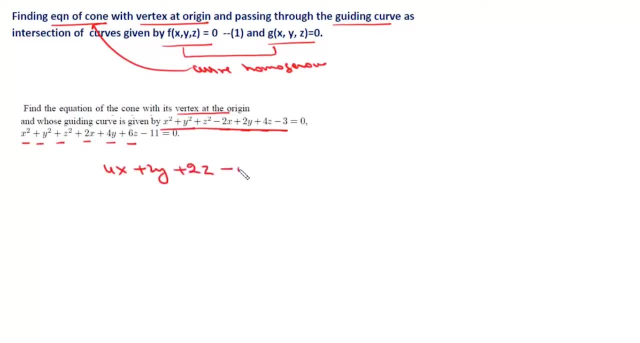 2z minus 8 equals 0, or that is 2x plus y plus z equals 4, and we can write this as 2x plus y plus z upon 4, and it is equal to 1.. Now, using this, we can make either of these two. 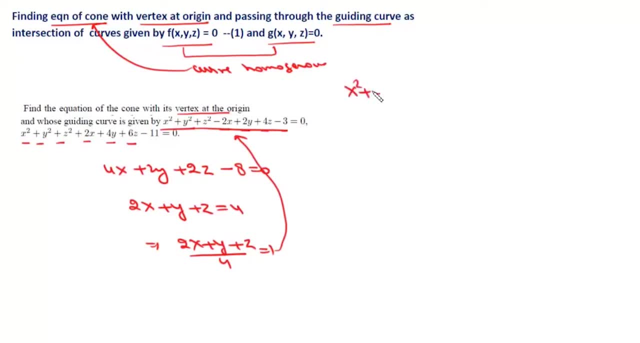 curves homogenous. So we can write this equation as: x square plus y square plus z square. here we have degree 2, and then plus minus 2x, plus 2y plus 4z, and here we need to increase this degree by 1.. So it will be multiplied with 1, and then minus 3 into 1 square equals 0.. 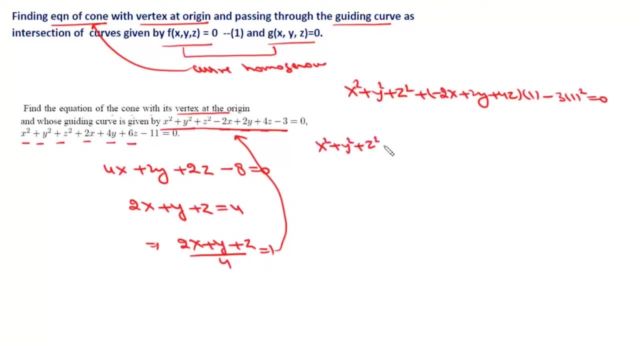 Now we can write this as x square plus y square plus z square, minus 2x plus 2y plus 4z into this 1, and this 1 is 2x plus y plus z upon 4 and minus 3, and here will be 2x plus y plus. 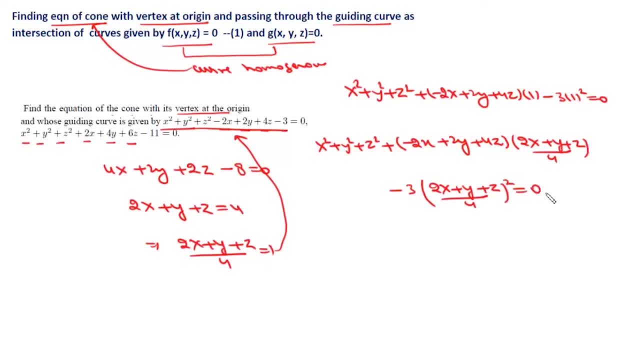 z upon 4 whole square and it will be equal to 0.. And if we simplify this equation, we will get this result as 12x square minus 21y square minus 29z square, Minus 28z square, Minus 18yz minus 12zx plus 4xy equals 0.. Which is the required equation of this code. 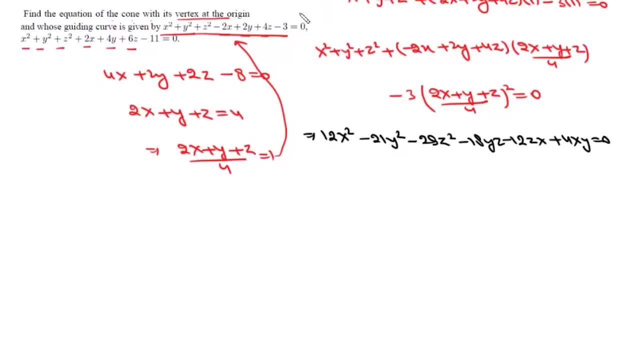 Now, another way to solve this equation is by taking a parameter t to make the curve homogenous. So we can write this first equation as x square plus y square plus z square minus 2xt plus 2yt plus 4zt Minus 2x. 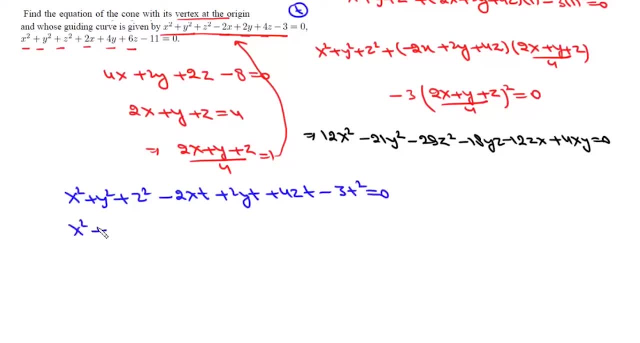 Minus 3t square equals 0.. And then we have x square plus y square plus z square plus 2xt plus 4yt plus 6zt minus 11.. t square equals 0.. Now again, we will subtract this first from second. 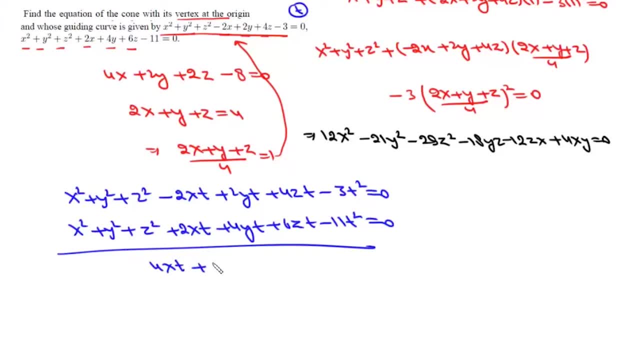 So we will get 4xt plus 2yt plus 2zt minus 3t, And then we have x square plus y square plus z square plus 2xt plus 4yt plus 3t Minus 3t. 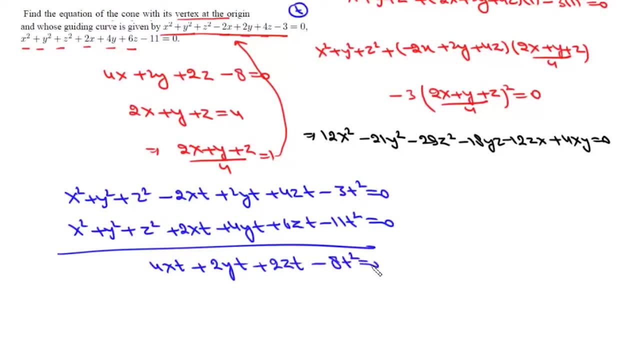 Minus 3t Minus 8.. t square equals 0.. So from here we will get this t as 2x plus y plus z upon 4. And if we put the value of t here, we will end up getting this same equation. 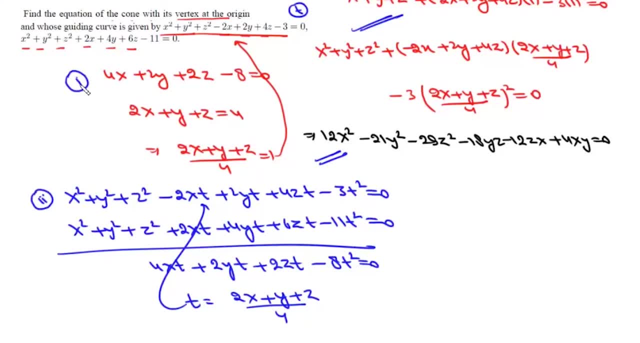 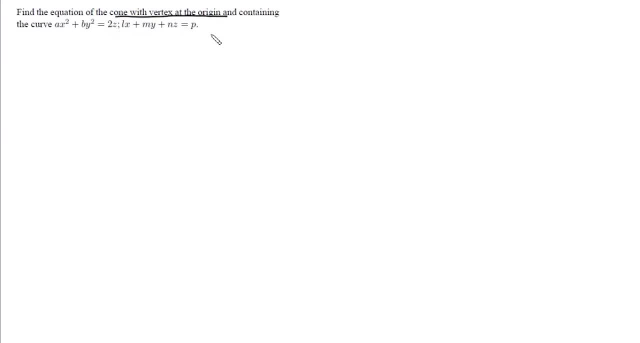 So that is second method of solving such questions. Now here the question is: find the equation of a cone with vertex at origin containing these two curves. Now here what we need to do is find the actual vertex. Now here what we need to do is we just need to make this curve homogeneous and it will. 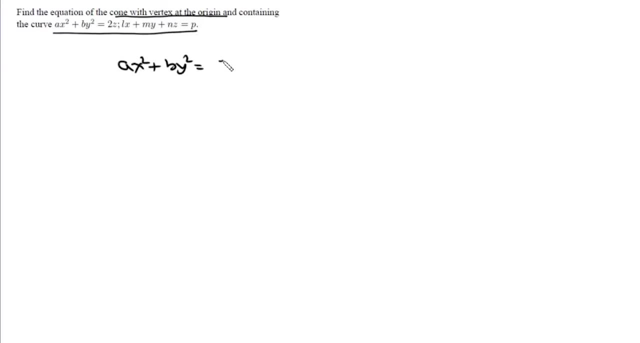 be given by ax square plus by square, and this is 2z, and we will multiply it with this one and we will get this one from lx plus my plus nz, upon p equals 1.. So this equation will be ax square plus by square plus 2z, that is lx plus my plus nz. 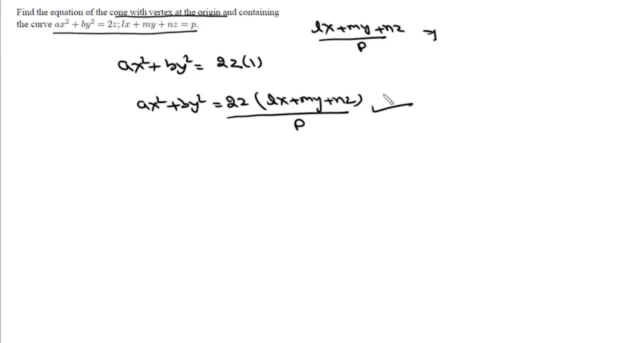 upon p, and this is the equation of required cone. Now here the question is: prove that this equation represents a cone and find its vertex. Now what we will do is we will assume it is some function f, and then we will find del f upon del x and we will put it equals to 0. we will find del f upon del y, we will put: 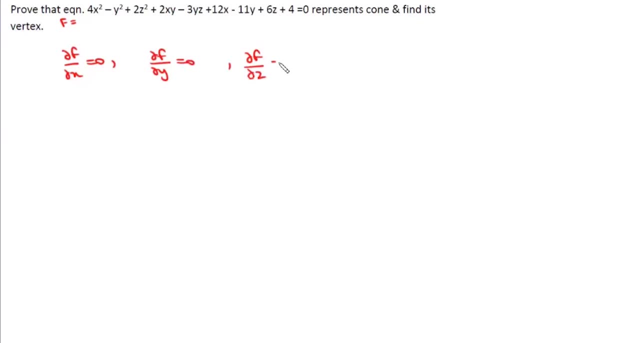 it equals to 0. and then del f upon del z and we will put it equals to 0 and we will solve these three equations to find vertex of this cone. Now we differentiate it with respect to the cone. So with respect to x, we will get this as 8x plus 2y plus 12 equals 0, which is 4x plus. 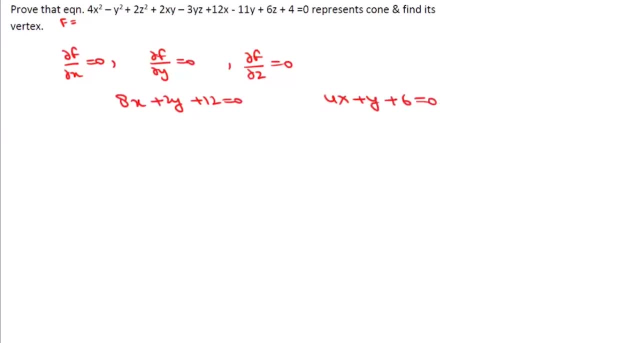 y plus 6 equals 0.. Now we differentiate it with respect to y, we will get minus 2y plus 2x minus 3z, minus 11 equals 0. So it will be 2x minus 2y minus 3z minus 11 equals 0.. 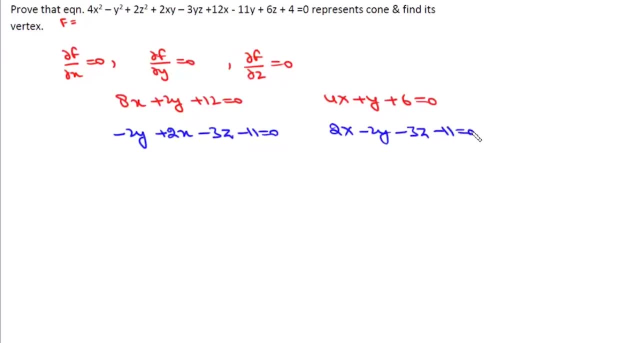 And then finally, we differentiate this equation with respect to z. we will get this as 4z minus 3y plus 6 equals 0, so that will be minus 3y plus 4z plus 6 equals 0.. Now from this second and third equation we will eliminate this y first, so we will multiply. 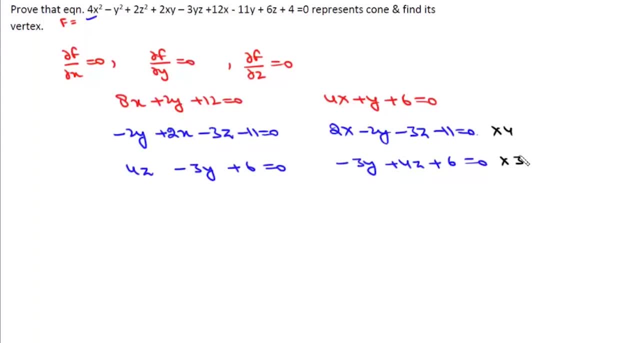 it with 4.. So we will add this with 3 and then we will get this as 8x. Now here it is 8y and minus 9y, so that will be minus 17y. Now this z will cancel. 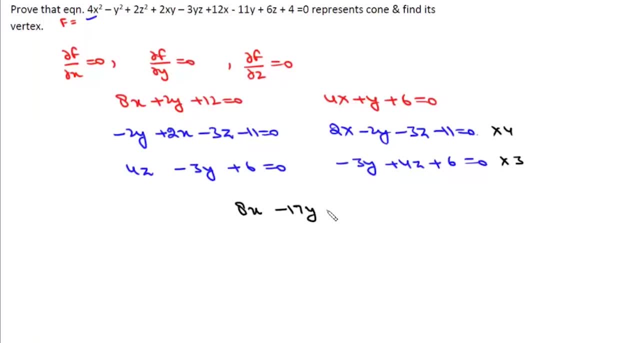 Now this is minus 44 and 18, which is minus 26, equals 0. and here we multiplied with 2, we will get 8x plus 2y plus 12, equals 0. Now we subtract this first from second, 8 and 8 will cancel, so we will get 19y plus. 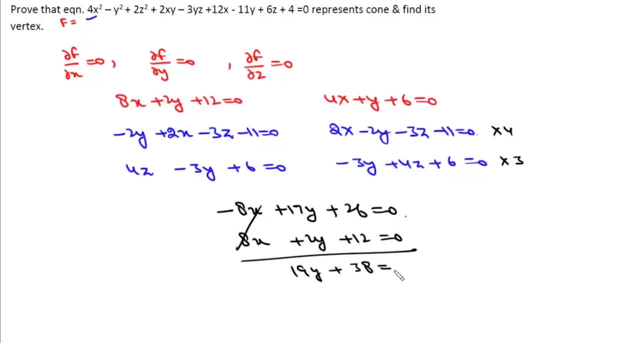 38 equals 0, so value of y is minus 2.. Now, if we put y as minus 2,, we will get x as minus 1.. And if we put y as minus 2 in this, we will get z as minus 3.. 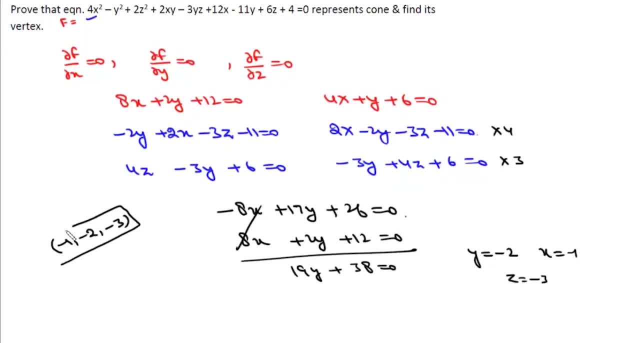 Vertex of this cone is at minus 1, minus 2 and minus 3.. And actually we have not verified this is the equation of a cone and for this what we will do is we will make this curve homogenous, which is say, 4x square minus y square plus. 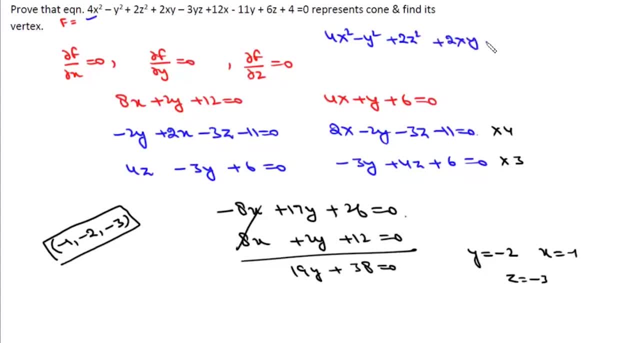 2z square plus 2xy minus 3yz plus 3z 12xt minus 11yt plus 6zt plus 4t square equals 0, and we will find del f upon del t and we will put it equal to 0.. 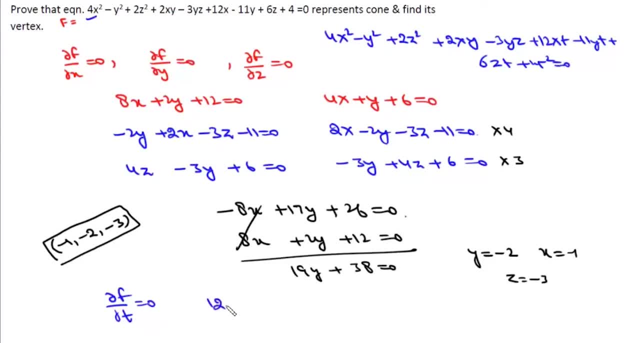 Now we will differentiate this with respect to t. we will get 12x minus 11y plus 6z plus 8t equals 0.. Now we put the value of xy and 2x z, we'll get minus 12 plus 22, minus 18 plus 8t equals 0.. Now this is 8t equals 8 and value of: 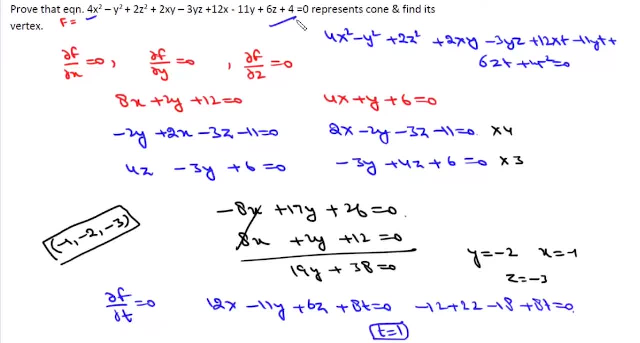 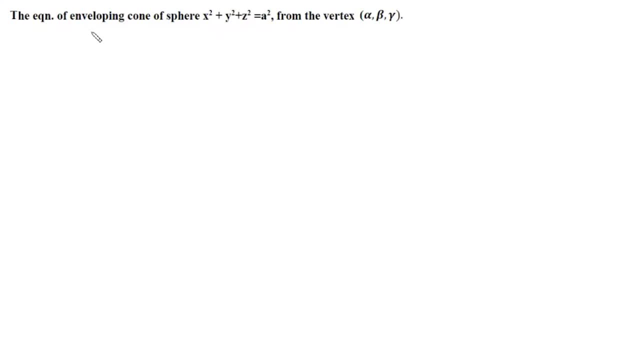 t is 1 and when we have value of t is 1 we'll get the same equation. So this equation it does represent equation of a cone. Now there will be questions on equation of enveloping cone of square. x square plus y square plus z square equals a square from the vertex alpha, beta and gamma. So 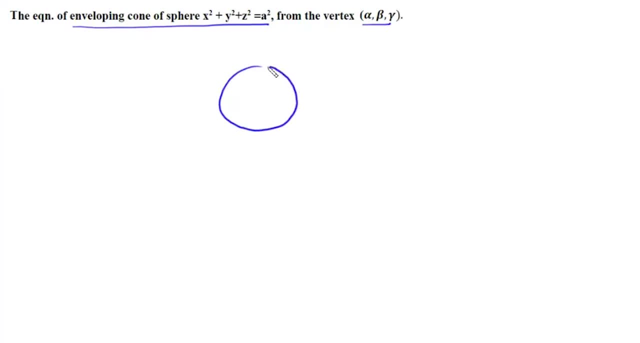 we have this square whose equation is: x square plus y square plus z square equals a square. and then we have this cone which envelops this square, and vertex of this cone is at alpha, beta and gamma. Now what we'll do is we'll take a point on this line, say this point. 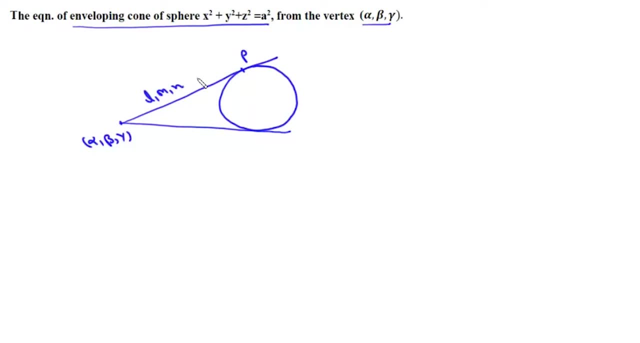 p and suppose direction ratios are l, m and n. We can write equation of this line as x minus alpha by l, y minus beta by n and z minus gamma by n and say it is equal to some lambda. Then we can coordinate of this point P as alpha plus l lambda, beta plus m lambda and gamma plus n- lambda. Now 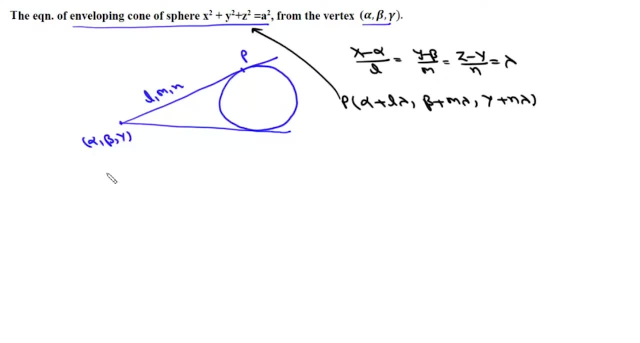 this point P, it lies on this sphere, So it satisfies its equation. So we can write: alpha plus l lambda square, beta plus m lambda square, plus gamma plus n lambda square, and it is equal to a square. Now we say: simplify this. We can write this equation as l square plus m square plus n square into lambda. 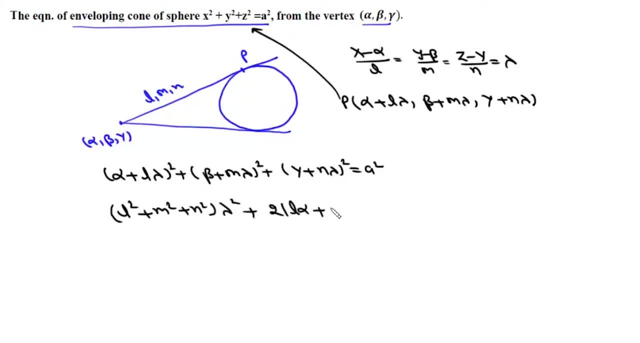 square plus 2 l alpha plus 2 m, beta plus 2 n gamma into lambda, and plus alpha square plus beta square plus gamma square minus a square. It must be equal to 0.. Now, since this line will be tangent to this square, it will have only one point of intersection. So this coordinate equation should have only one real root. That means value of D. it must be equal to 0.. Now we put b square equals 4ac. we will get 4l alpha plus m beta plus n gamma whole square and it will be equal to 4ac. So it will be 4l square plus m square plus n square into alpha square plus beta square plus m square. 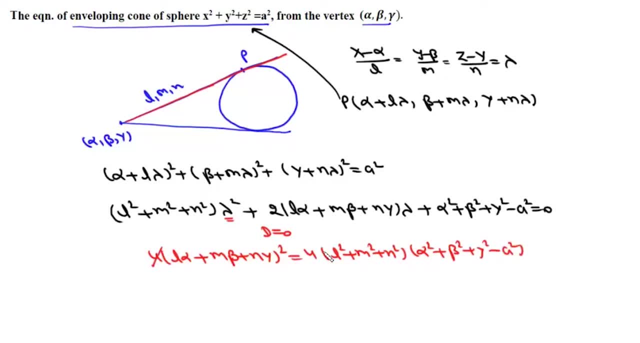 Now this 4 and 4 will cancel. Now we need to eliminate l, m and n, and what we can also do is we can multiply everything with lambda, So we can write lambda l, alpha, lambda m, beta, lambda n, gamma square, So it is lambda square here and here we can write lambda l square, lambda m square plus lambda n square, and this is alpha square plus beta square plus gamma square, minus a square. 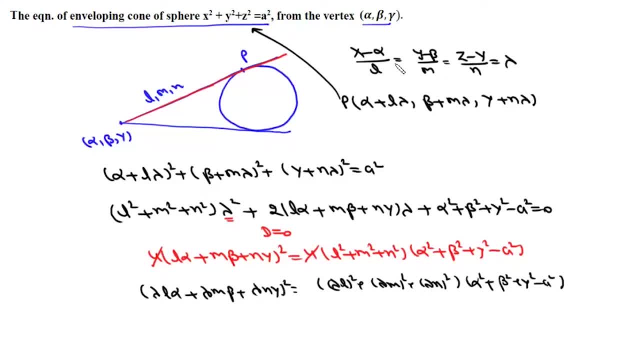 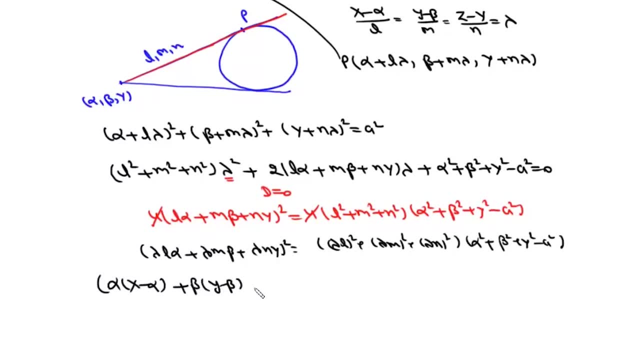 square. Now lambda L, it is nothing but x minus alpha. So we can write this as alpha into x minus alpha, plus beta, into y minus beta and plus gamma into z minus gamma whole square, And it'll be equal to x minus alpha square, y minus beta square and z minus gamma whole square, And it'll be equal. 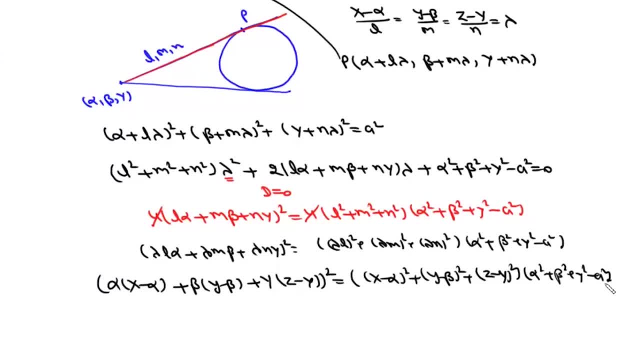 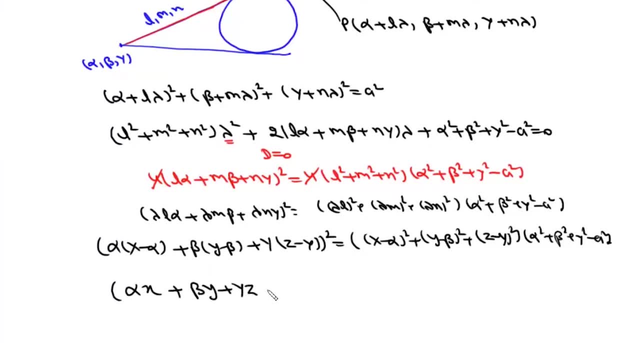 to alpha square plus beta square plus gamma square minus a square. And if we simplify this, it'll simplify to alpha x plus beta, y plus gamma, z minus a square, whole square, And it'll be equal to x square plus y square plus z square minus a square, And it'll be alpha square plus beta square. 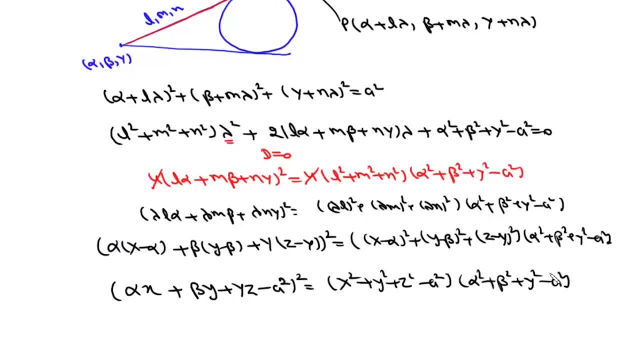 plus gamma square minus a square. And if you are familiar with concepts in conic sections, then we know that equation of pair of tangents is given by S? S1 equals T square and this form itself is S? S1 and this is T square. So we can also solve this question directly by using this concept of S? S1. 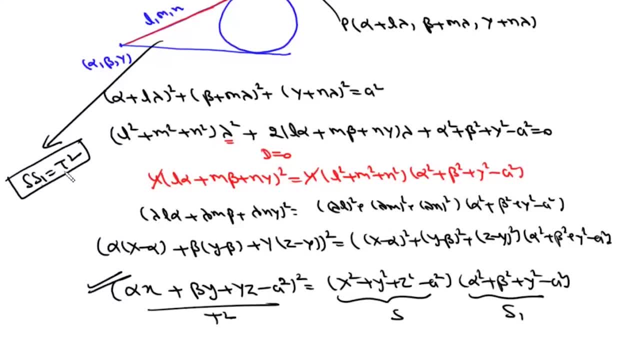 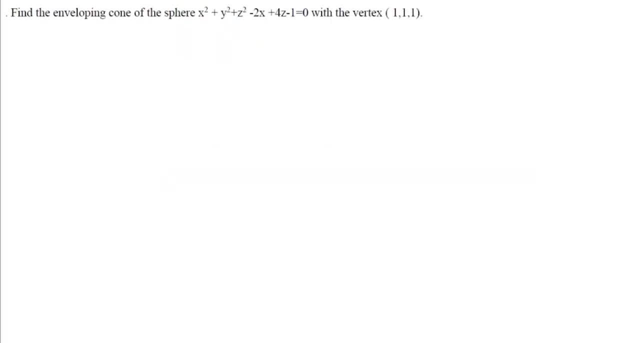 equals T square. We have already discussed how to find S1 and T in one of the previous videos in conic sections, So I'll put the link to that video in the description below. Now here the question is: find the enveloping cone of this sphere with vertex at 1, 1, 1.. Now, if we find T, 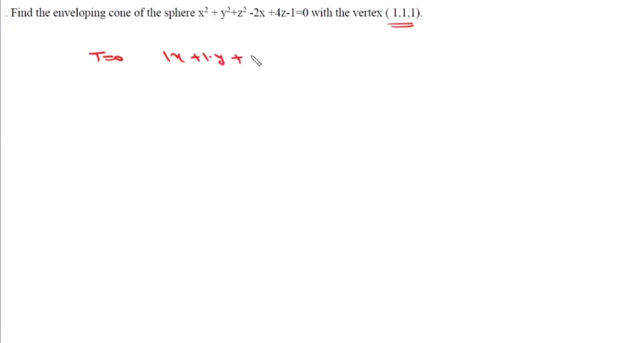 equals 0, T equals 0 will be 1 X plus 1 Y, 1 Z minus X plus 1 plus 2. Z plus 1 and minus 1 equals 0. So this equation will be now this: X and X will cancel. We'll get this as Y plus 3 Z. 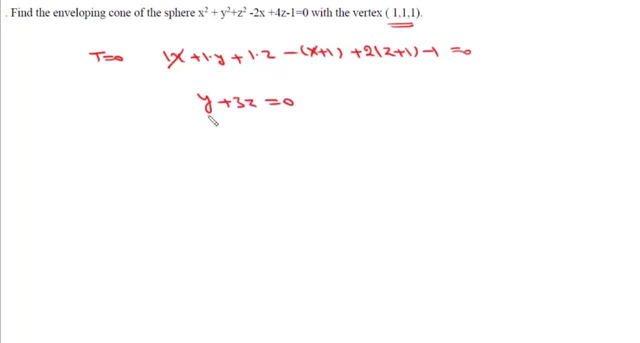 equals 0.. So now we have R, T, and S is basically the same equation. So this S is X square plus y square plus z square minus 2x plus 4z minus 1, and then s1 is this value if we put x, y. 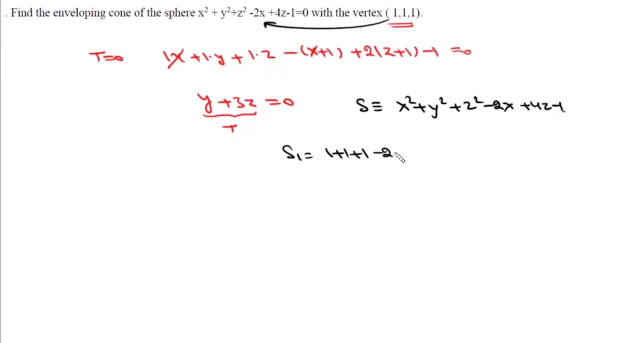 and z in this equation. so we'll get 1 plus 1 plus 1 minus 2, plus 4 minus 1 and there will be 4. so equation of this enveloping cone will be: s: s1 equals t square. now s is x square plus y square. 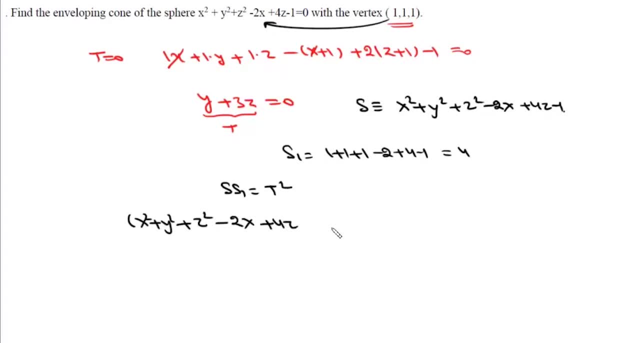 plus z square minus 2x plus 4z minus 1 into 4, and it'll be equal to y plus 3z whole square. now this is 4x square plus 3y square minus 5z square, and then it'll be minus 6yz minus 8x. 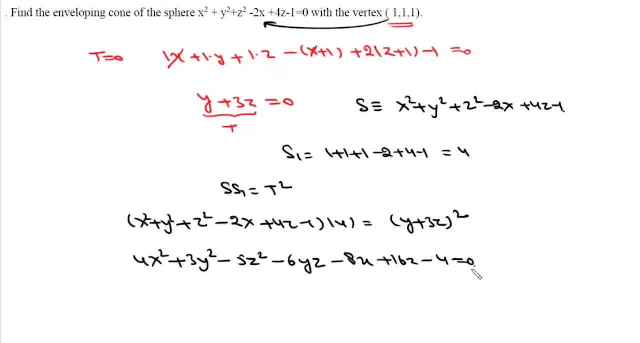 plus 16x, z minus 4 equals 0, and that is the equation of enveloping cone of this sphere.